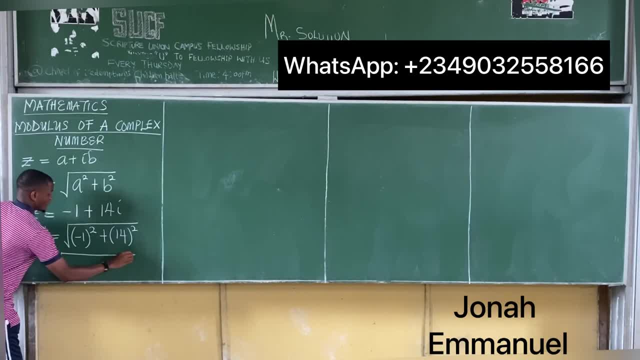 So here it's equal to the square root of minus 1 squared. So minus 1 squared is 1 plus 14 squared. Let's get this done: 14 squared is equal to 196.. 14 squared, This is equal to the square root of 197.. 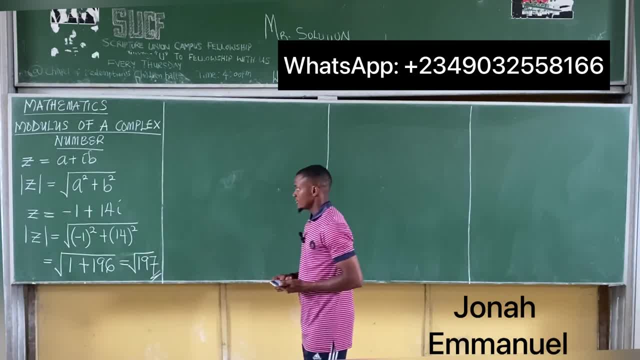 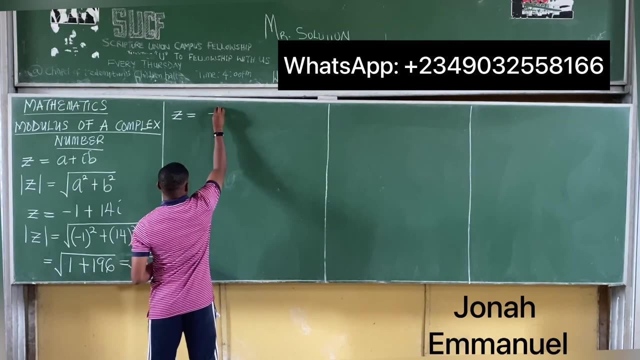 So hence, the modulus of Z is equal to root 197.. So this is how we get modulus of a complex number. A second example: Let's say we have the complex number Z being equal to minus 1 minus I, And I'm asked to find the modulus of Z. 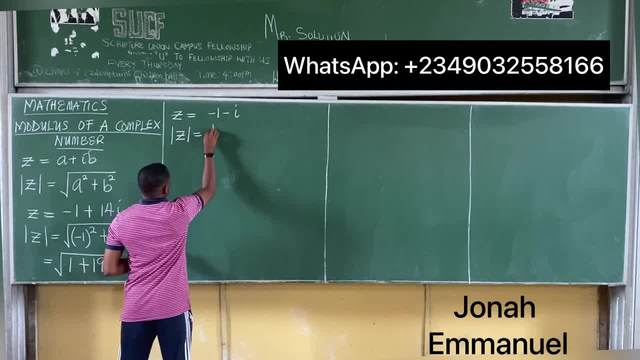 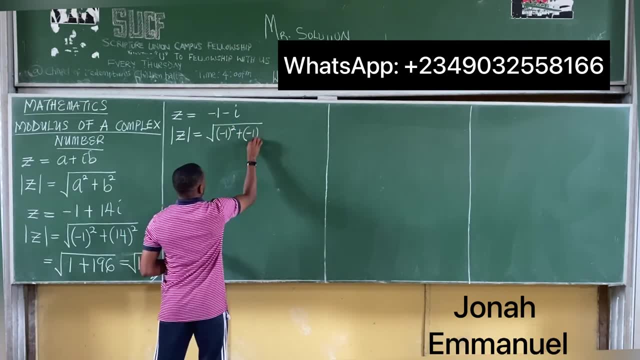 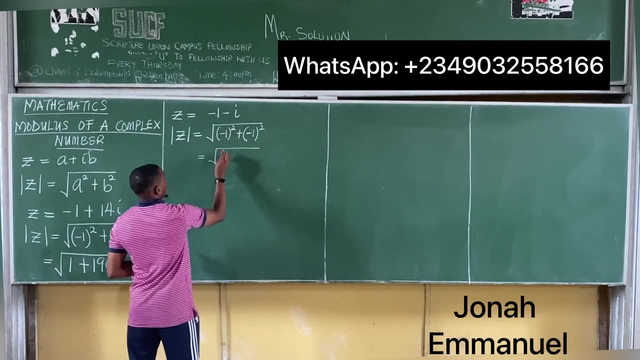 The modulus of Z. that Z is equal to the square root of this term, minus 1 squared, plus the coefficient here is minus 1 all squared. If I work on this, this is equal to the square root of minus 1 all squared. 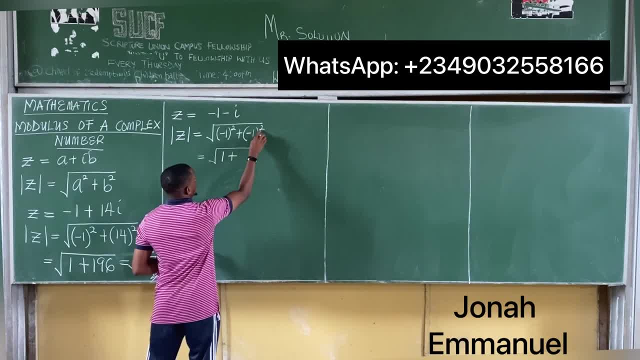 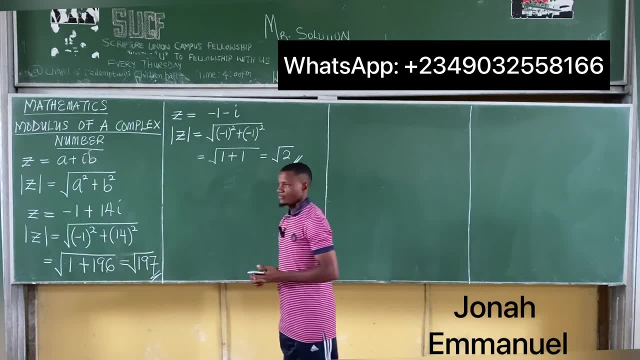 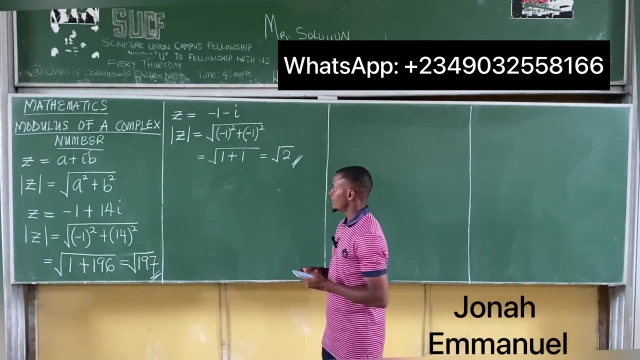 Gives you positive 1 plus minus 1. all squared Gives you positive 1, and that's equal to the square root of 2.. So this is how we get the modulus of a complex number. Alright, let's proceed. So take a sample problem on modulus of a complex number and see how we can get this done. 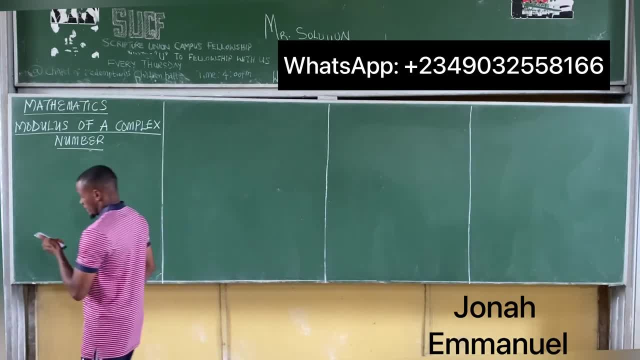 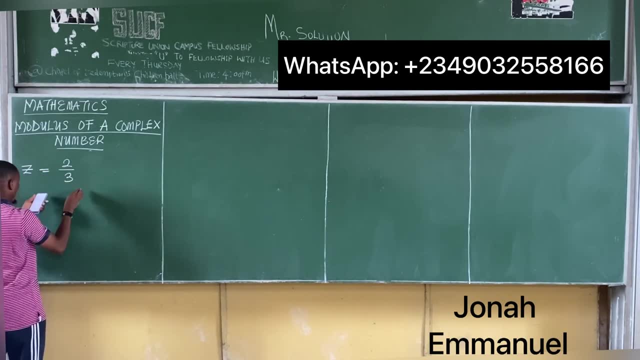 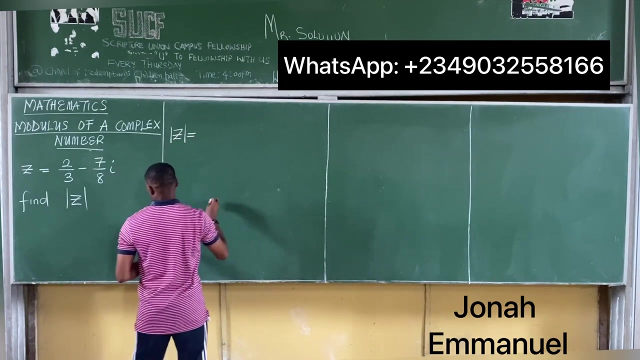 Alright. so this question says: This question says: If Z is equal to 2 over 3 minus 7 over 8, I find the modulus of Z. So this is as simple as we said. the modulus of Z would be equal to the square root of the first term there. 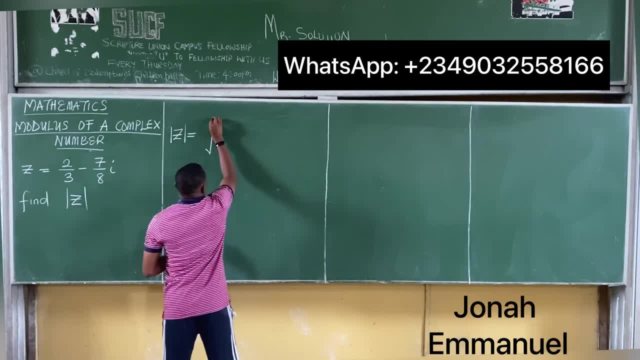 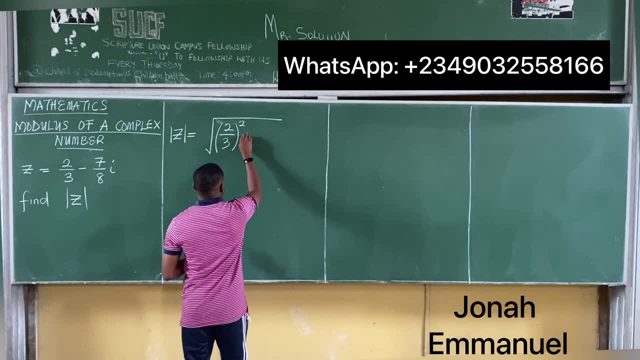 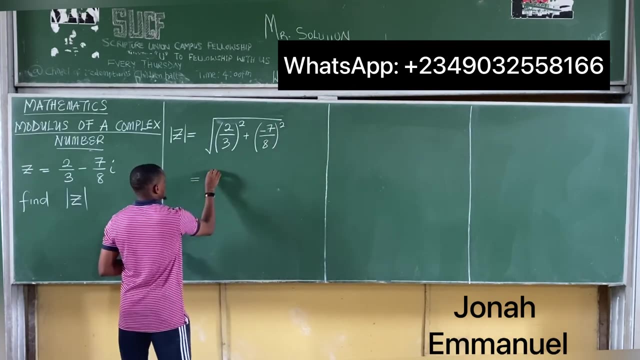 Now the square root of the first term there: 2 over 3 all squared, plus the next term there is minus 7 over 8 all squared. This is equal to the square root of 2 squared is 4, 3 squared is 9 plus minus 7 all squared is 49 all over. 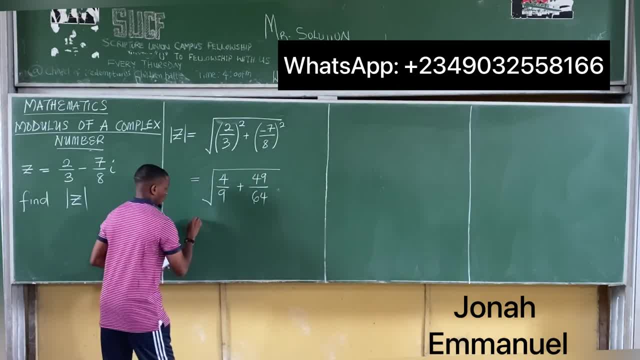 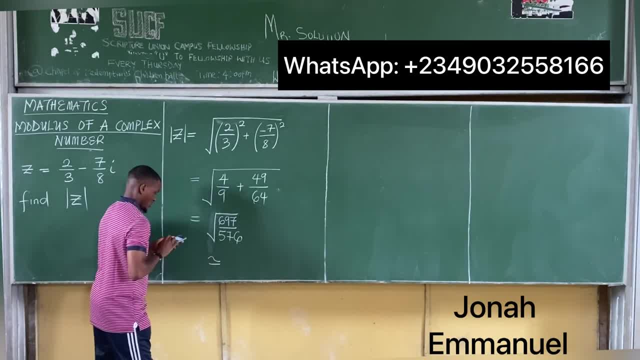 So that's about the square root of 6,, 9,, 7 all over 5.. So I have this. Perhaps in 2DP I would have. perhaps in 2DP I would have 1.10 or less than 1DP 1.1.. 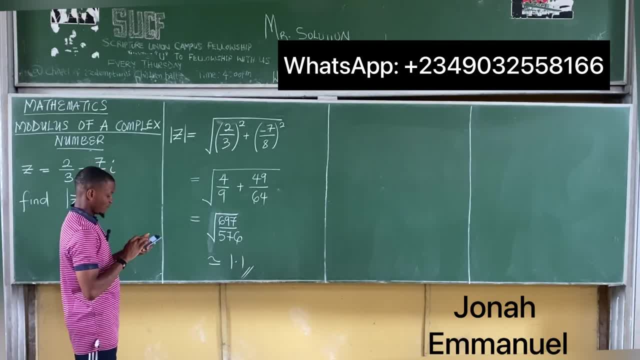 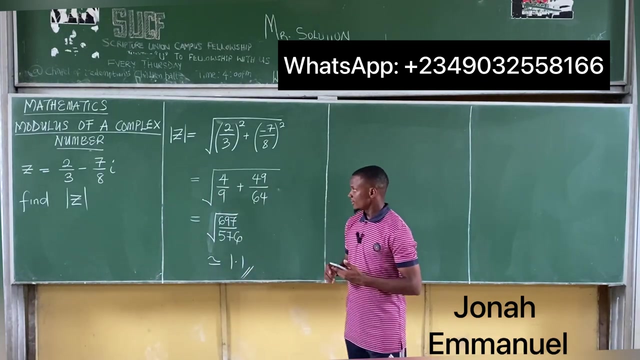 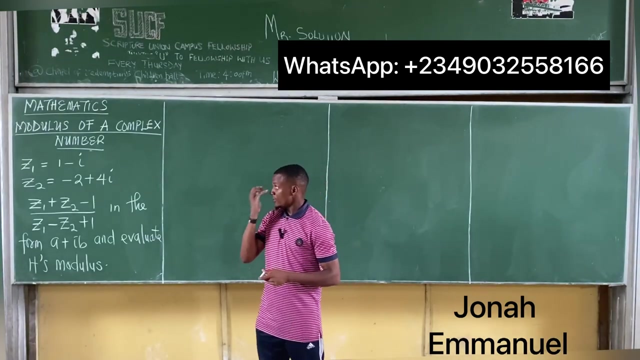 So that's your answer. So this is how you get the modulus of, of of of a complex number. all right, so that is this how this is done. we take one more example on this and they'll do something else, all right. a final question on models of vectors or on models of the complex. 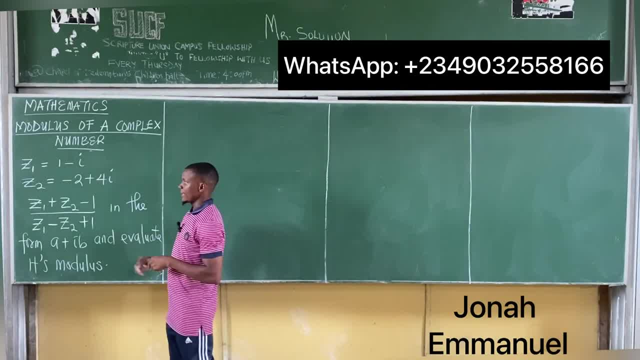 number. it says: if z1 is equal to 1 minus i and z2 is equal to minus 2 plus 4i, evaluate z1 plus z2 minus 1 all over z1 minus z2 plus 1 in the form a plus ib. 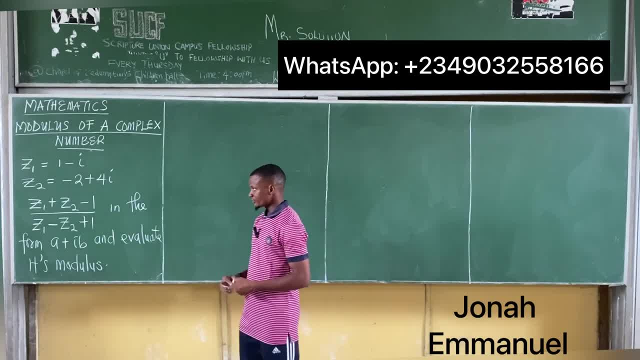 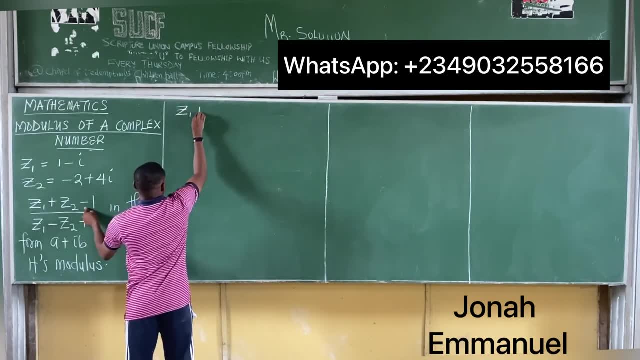 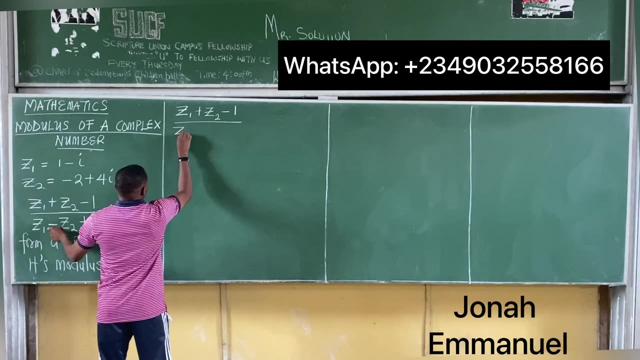 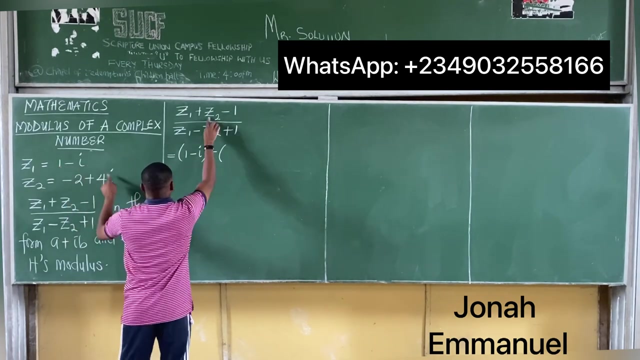 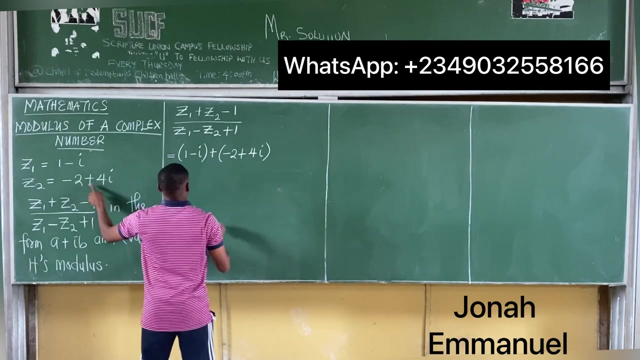 and evaluate its models. my first task here is to get this expression z1 plus z2 minus 1 all over z1 minus z2 plus 1. if i substitute values, z1 is equal to 1 minus i, plus z2 is minus 2 plus 4i. then next up: plus minus 1, so minus 1 all over z1. 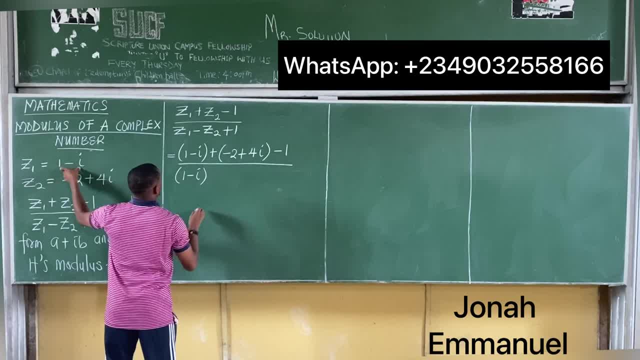 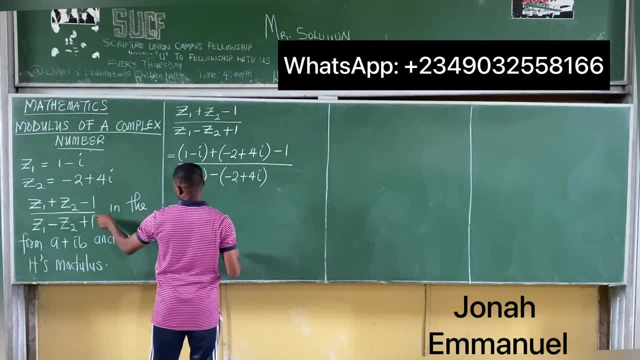 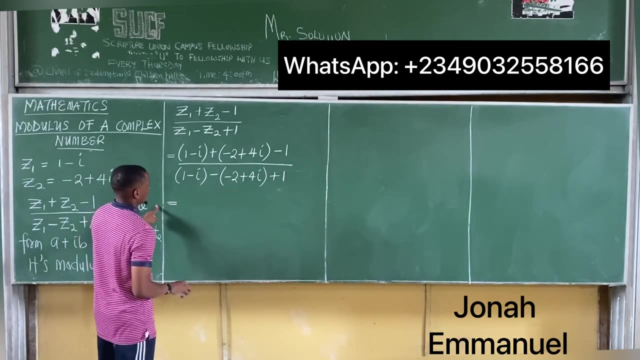 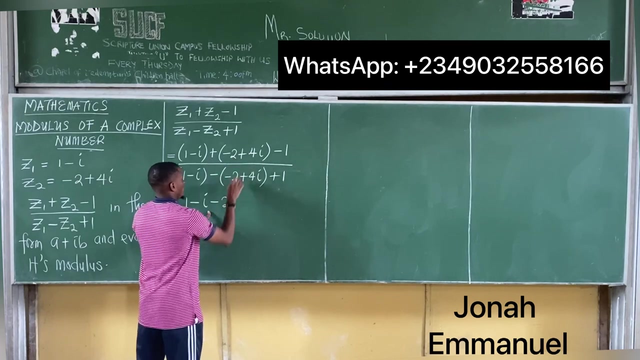 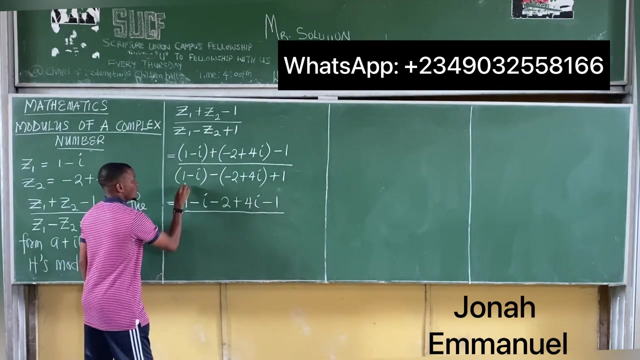 1 minus i, minus z2, minus 2 plus 4i, then plus 1, so plus 1. i have this. so evaluate this. what do we get? i'm taking off the brackets. i have 1 minus i plus minus is minus 2, plus plus is plus 4i. finally, minus i all over, 1, minus i, minus minus is plus 2. 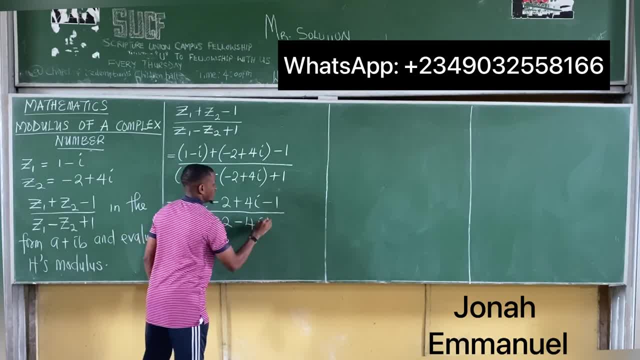 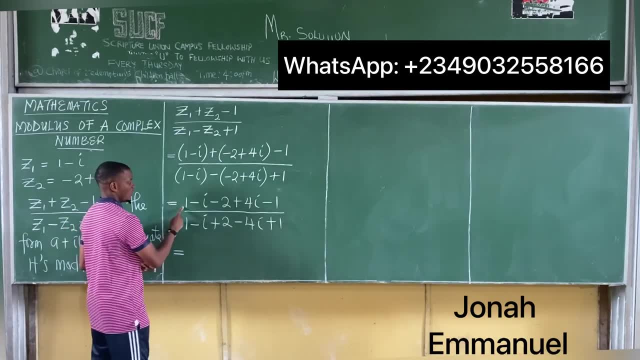 minus plus is minus 4i, then plus 1. so i have this working on. this is equal to take out the real parts: 1 minus 2. minus 1 minus 1 gives you minus 2, so all the real parts in my numerator gives me minus 2. take out the imaginary parts minus. 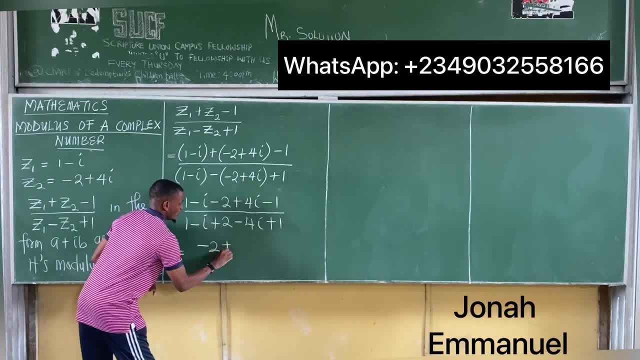 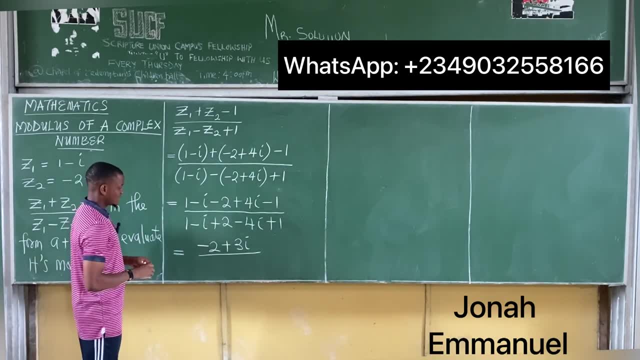 minus i plus 4i gives you plus 3i all over for denominator. take out the real parts: 1 plus 2, that's um 3 plus 1, that's 4 minus i. minus 4i for imaginary part gives me minus 5i. 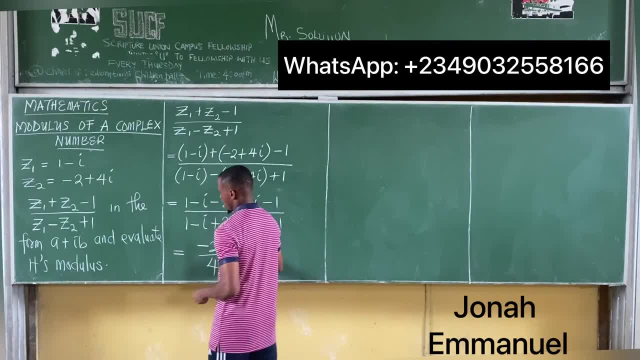 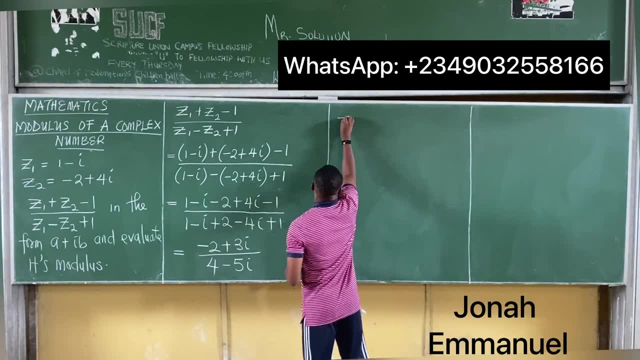 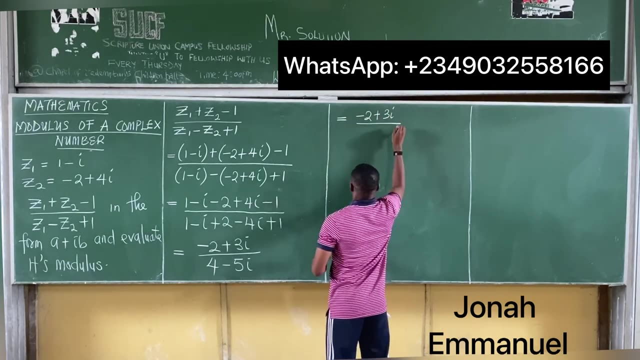 so i have this value, but we have to express this one here in this form: a plus ib. so hence, if i have this, i'll have to rationalize, and that's equal to rationalizing. we have minus 2 plus 3i, all over 4 minus 5i. we have to rationalize: simply multiply numerator by the conjugate of denominator. 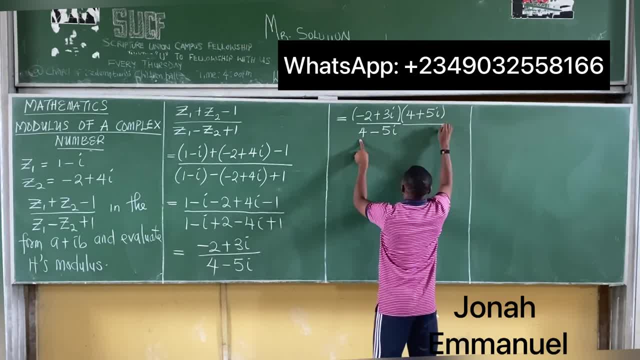 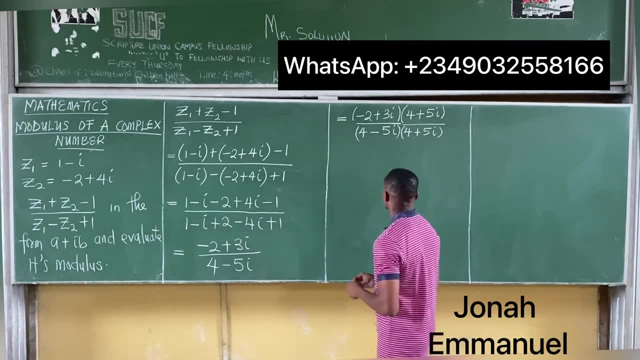 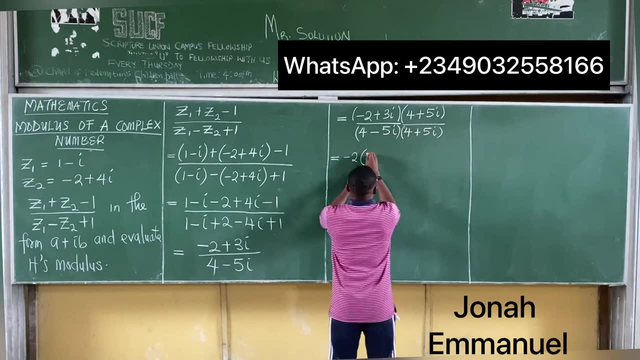 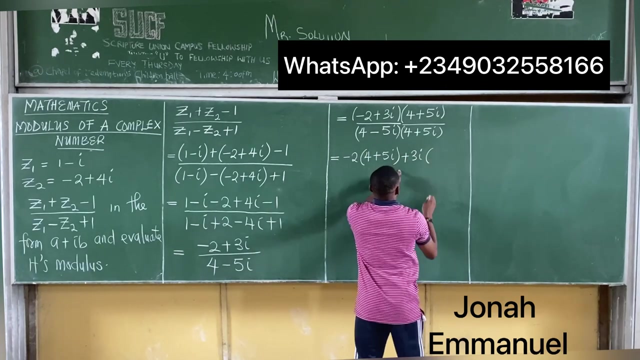 4 plus 5i all over. this one here: 4 plus 5i, so i have this one here. so this is equal. to use the first term here minus 2. multiply everything here: 4 plus 5i. use the second term plus 3i. multiply everything here: 4 plus 5i, so we have this here all over. use the. 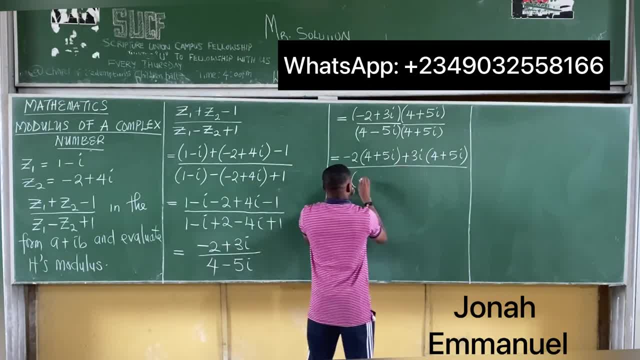 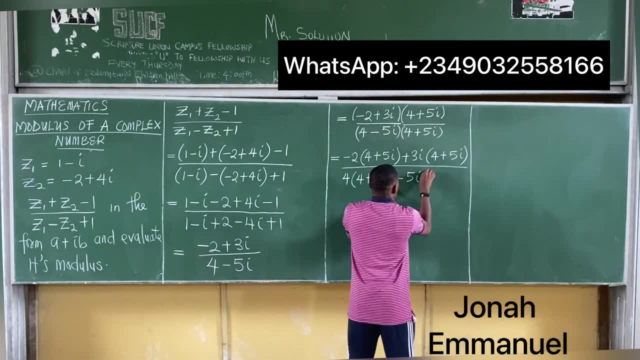 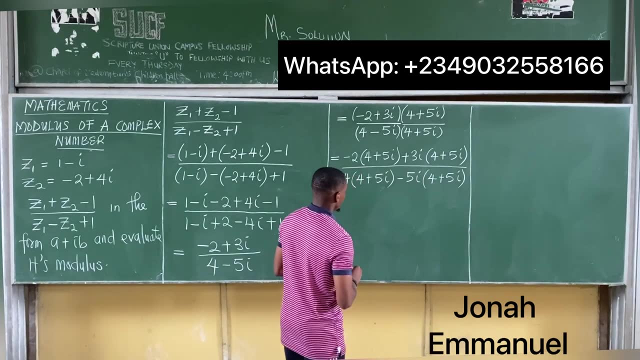 first term here: 4. multiply everything here 4 plus 5i. second term here: minus 5i. multiply everything here: 4 plus 5i. so i have this all right. so in expansion, what do you have? expanding this: minus 2 times 4 is minus 8.. Minus times plus is minus. 2 times 5 is 10.. Bring down your i. 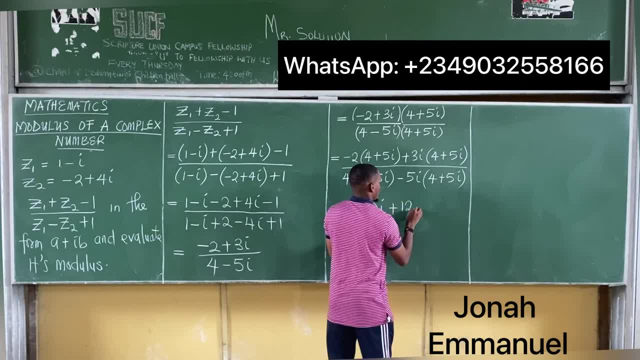 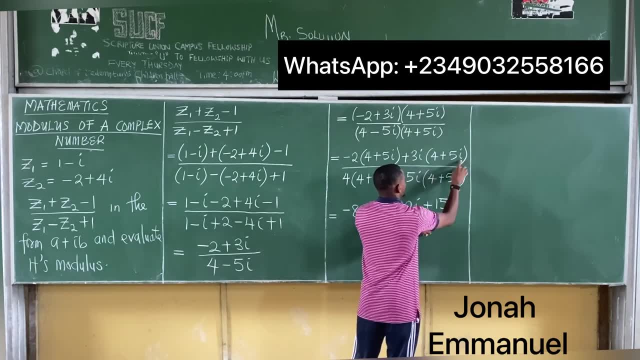 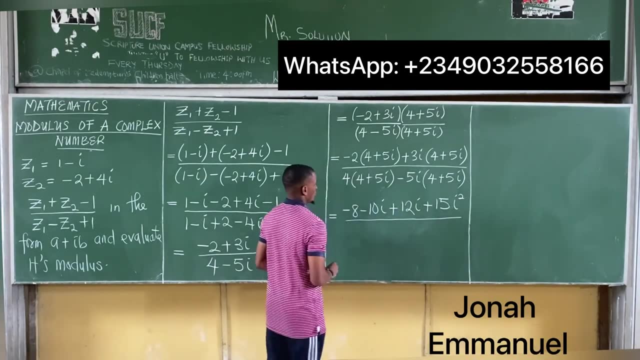 Plus 3 times 4 is 12.. Bring down the i Plus plus is plus 3 times 5 is 15.. i times i is i squared. So we have this all over For denominator. we have 4 times 4, 16.. 4 times 5i gives you. 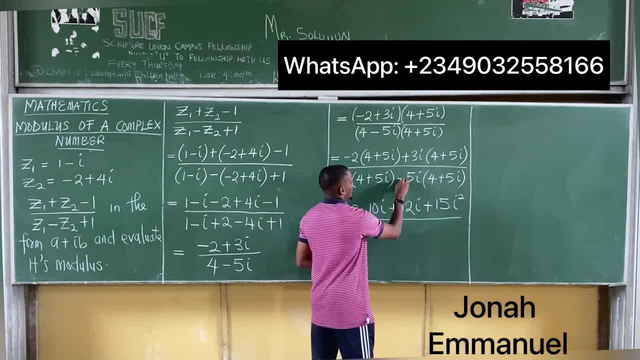 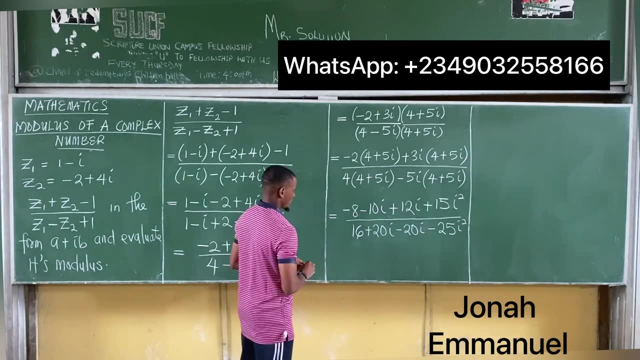 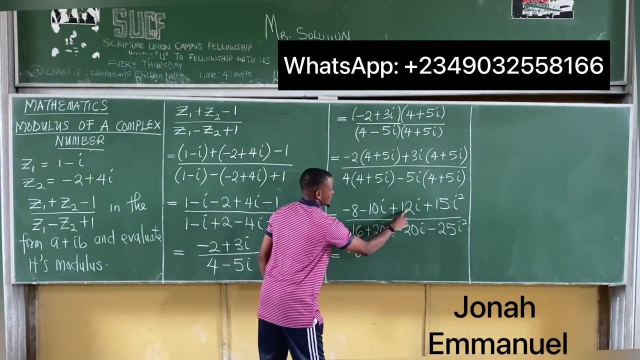 20i Minus 5 times 4 is minus 20i. Minus times plus minus 5 times 5, 25.. i times i, i squared, So I have this. So work on this. This is equal to: I have here as minus 8.. Minus 10 plus 12 is plus. 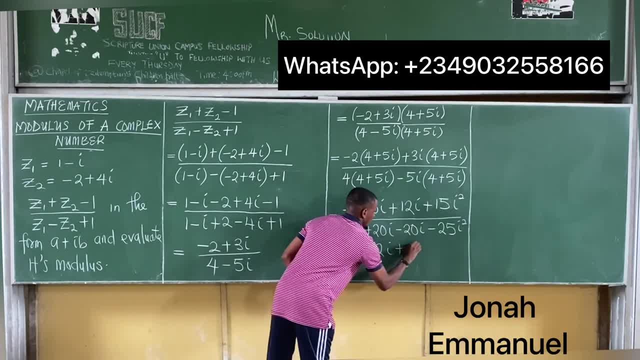 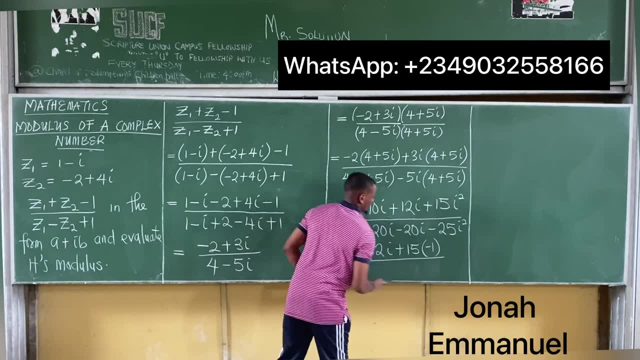 2i plus 15 into i squared. We said the value of i squared is minus 1.. All over, this is 16. Plus 20 minus 20.. They will cancel each other, So I'm left with minus 25.. 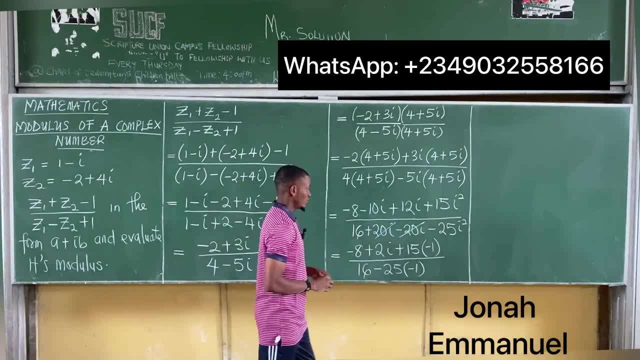 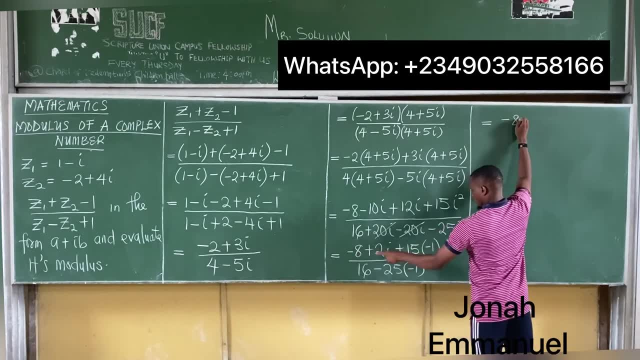 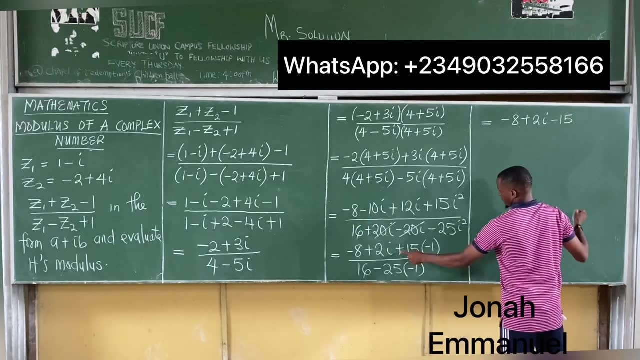 i squared, we said is minus 1.. All right, So this is equal to: I'm having minus 8 plus 2i, plus minus minus 15.. That's plus 15 times minus 1.. Minus 15, all over 16.. Minus 25 times. 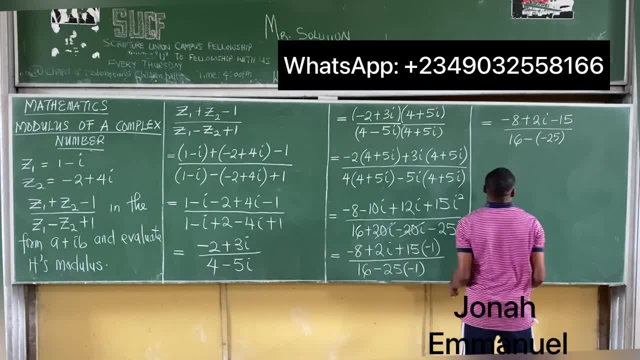 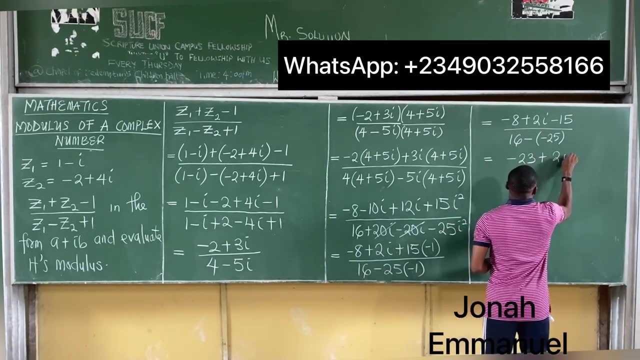 minus 1 is minus 25.. So I have this. If I work this out, take out the real parts here: Minus 8 minus 15.. That's about minus 23 plus 2i all over 16.. Minus minus is plus. It becomes 16 plus 25.. That's 41.. So hence, 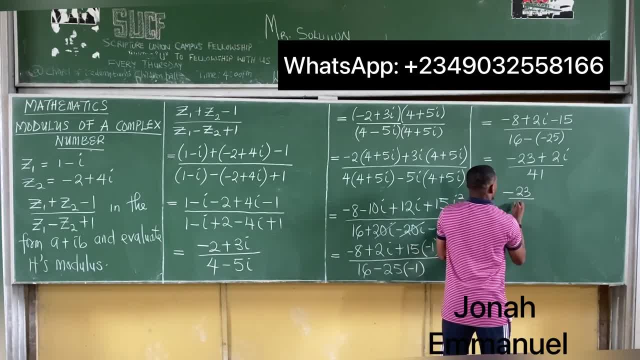 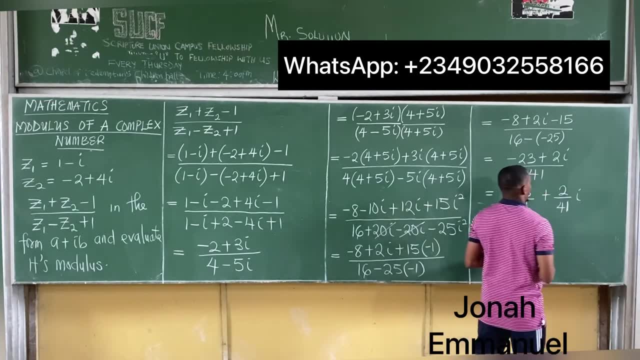 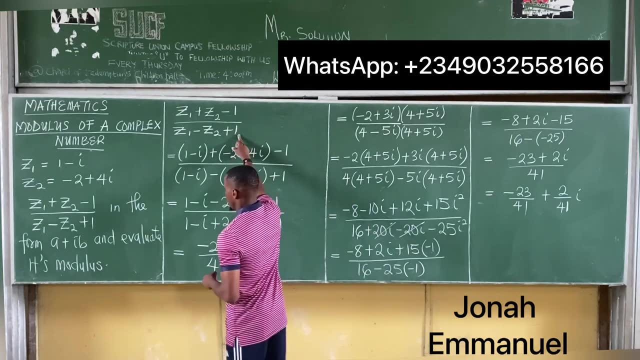 this will be equal to minus 23 over 41.. Plus 2 over 41 all into i. So we've gotten the value of this. Our next task- or we've expressed this one here in the form a plus ib, which is this: Our next task is to get. 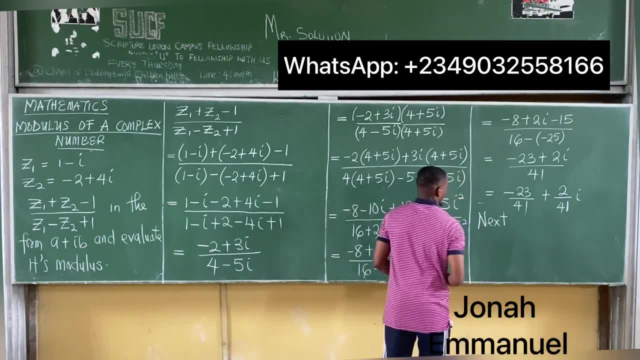 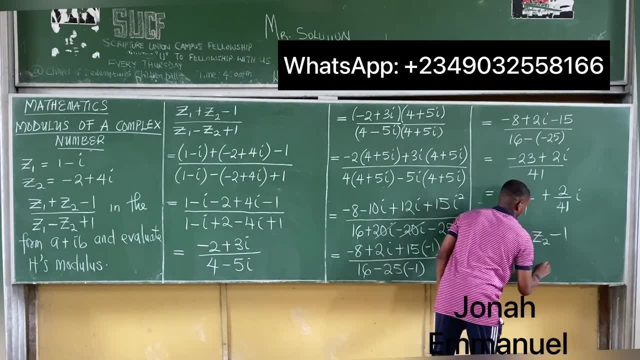 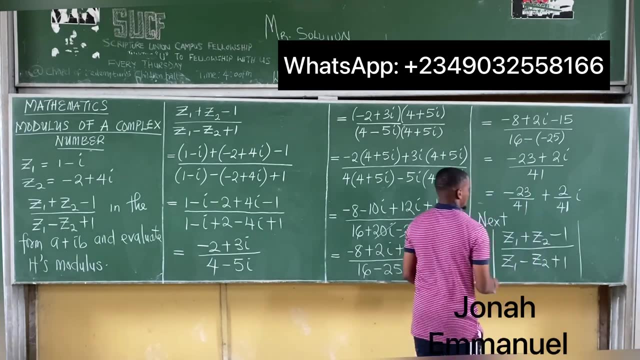 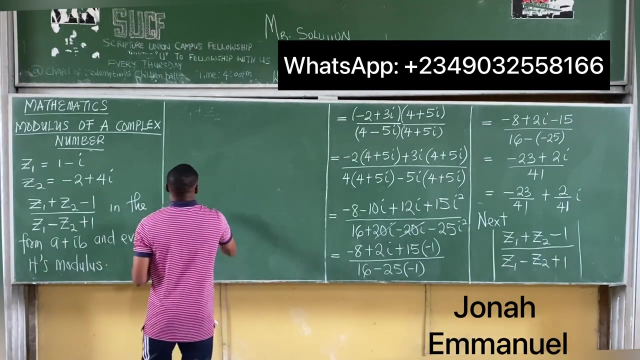 to next up, We have to find the modulus. So find the modulus of z1 plus z2 minus 1, all the modulus of z1 minus z2 plus 1.. Let's evaluate the modulus of this. All right, So the modulus would now be equal to the square root of minus 23 over 41 squared. 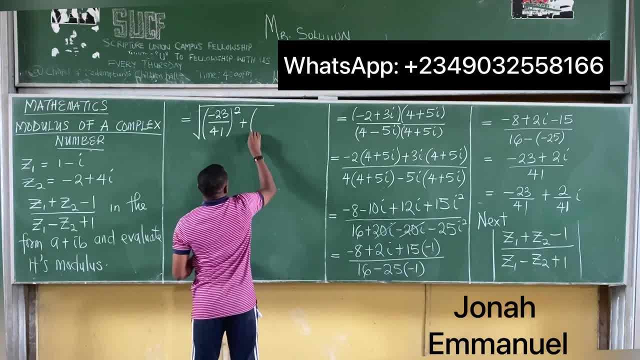 plus 2 over 41, plus the square root of minus 23, all over 16.. So we've done that. We're now going to ask for the modulus. So the modulus of z2 plus 1 minus the square root of minus 0 is equal to minus 3 over 2.. Next we have to find this. So let me do a little bit of. 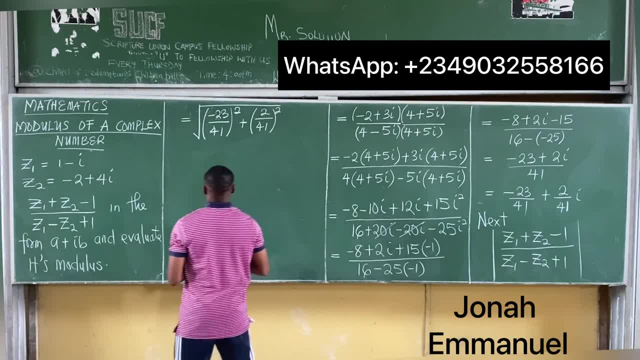 z1.. The modulus of this. So let me do a little bit of z2 plus 1 minus z2 plus 1 minus z3.. So here let's R squared, Let's get this done. This is equal to. let me get my calculator. 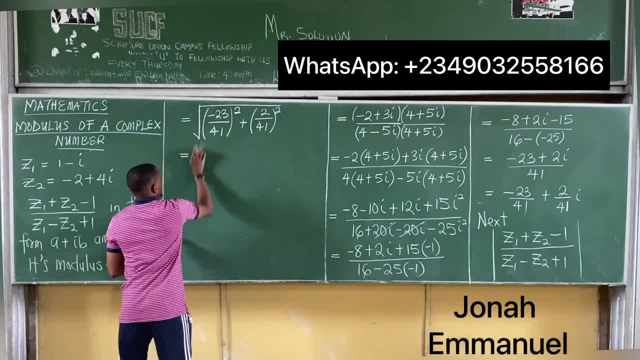 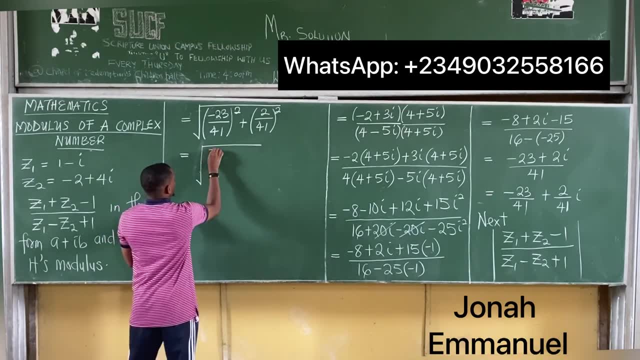 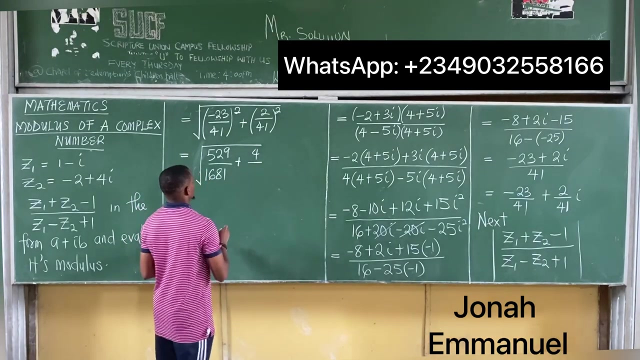 That's equal to the square root. Make this bigger. Square root of 23 squared is 529. all over 41 squared is 1681.. Plus 2 squared is 4, all over 41 squared is 1681.. If I sum this up, same denominator I'm having. 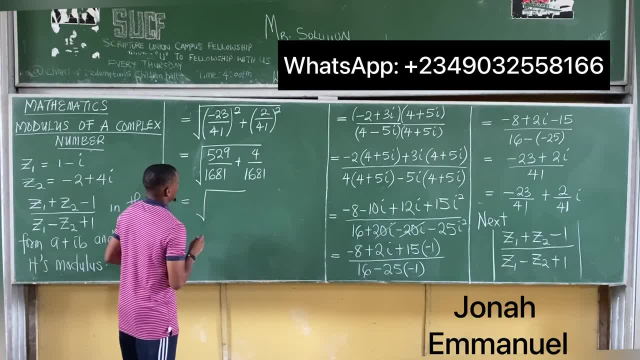 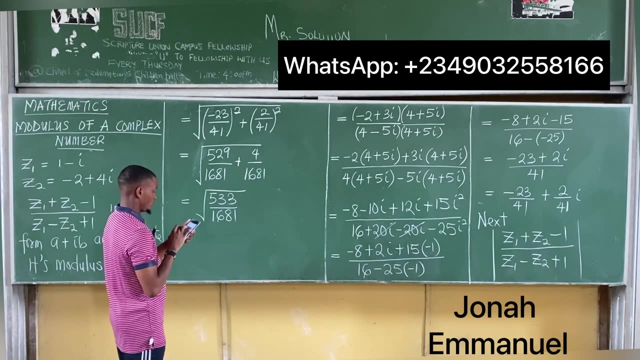 the square root of 533 all over 1681.. So I have this one here: Let's devalue Square root of 533 all over 1681.. So that's about: let's see if we can get this one here in. 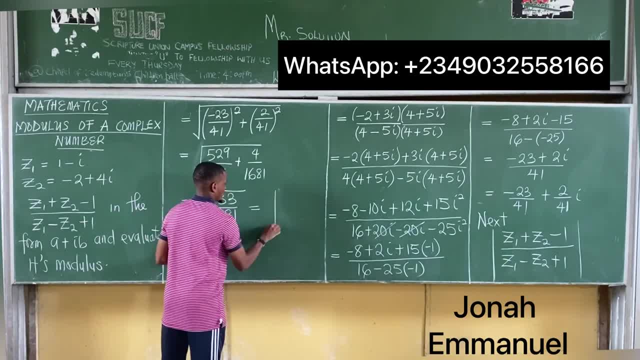 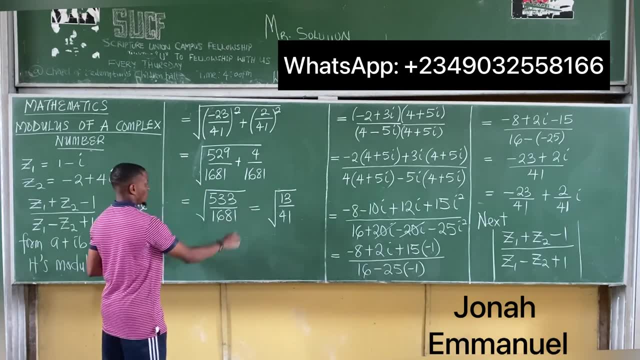 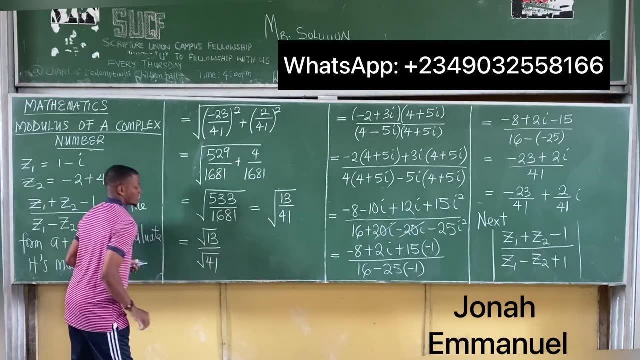 third form. In its simplest form, this is equal to the square root of 13 over 41. So if I have this now we can see we write this as being equal to root 13 all over root 41. So I have this one here Now we know. 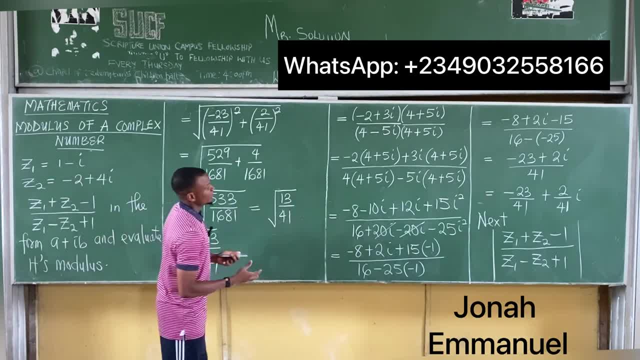 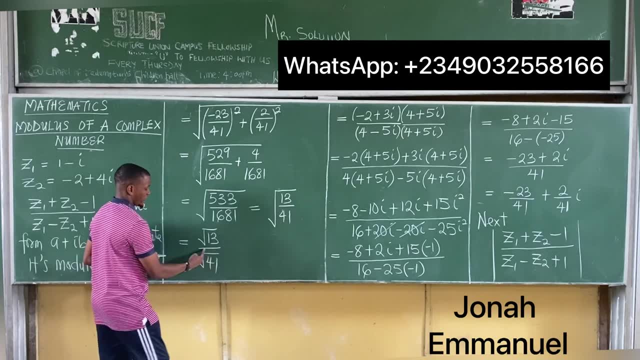 fully well that we cannot leave. just like we cannot leave the denominator of a fraction as a complex number, we cannot also leave the denominator of a fraction as a third. So in this case I'll have to rationalize the third. So, rationalizing the third. 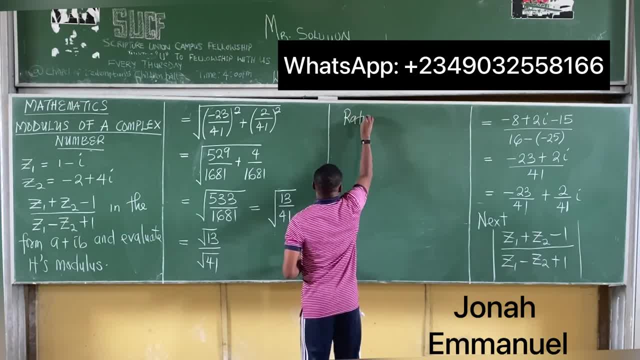 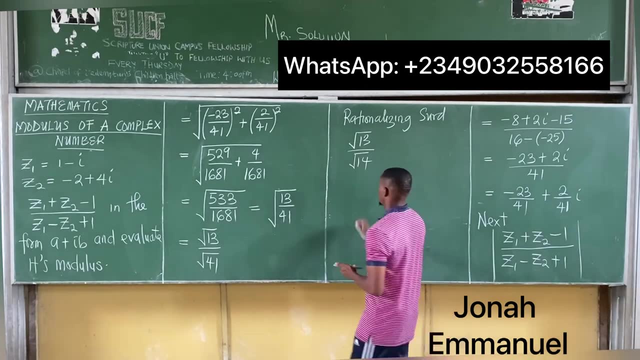 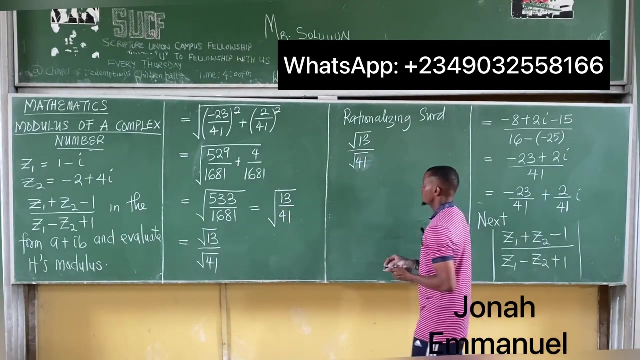 So let's rationalize third. Rationalizing third: would have that, would have that, would have that: Root 13 all over root 14.. To rationalize a third: sorry, all over root 41.. To rationalize a third in this form, you simply multiply. 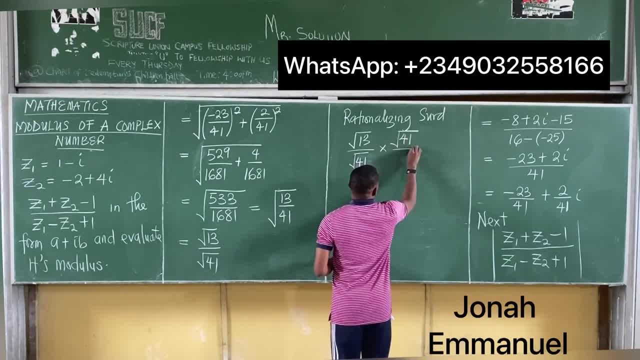 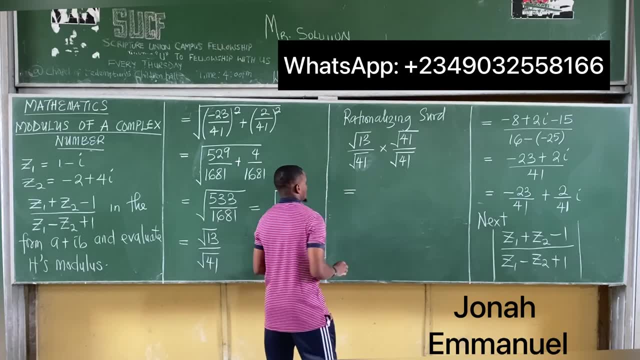 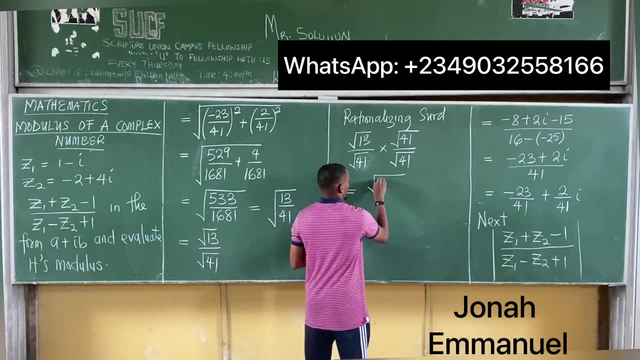 numerator and denominator by the denominator. That is so. multiply numerator and denominator by denominator, That's equal to roots 13 times. That's equal to roots 13 times. That's equal to roots 13 times 41 is 5, 3, 3. 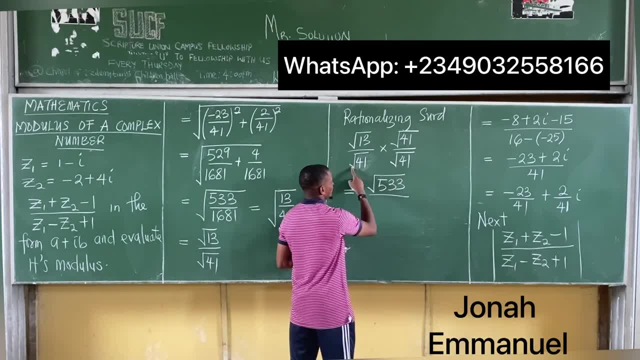 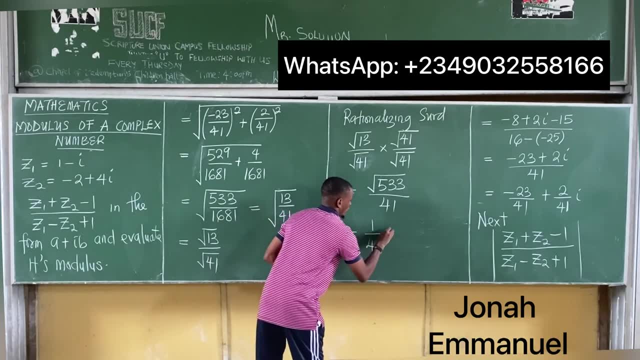 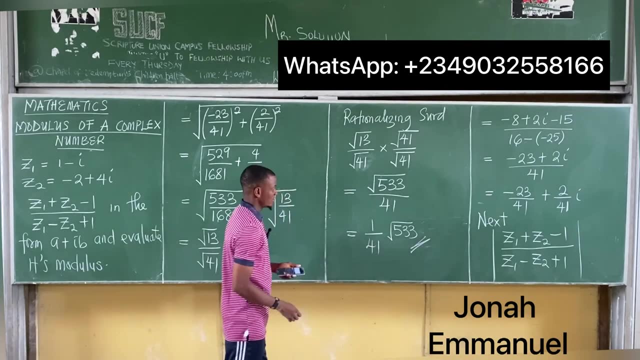 all over. root 41 times root 41 gives you 41. Hence, my answer is equal to 1 over 41. root 5, 3, 3.. These two are the same thing, Alright, So this is how we solve this. 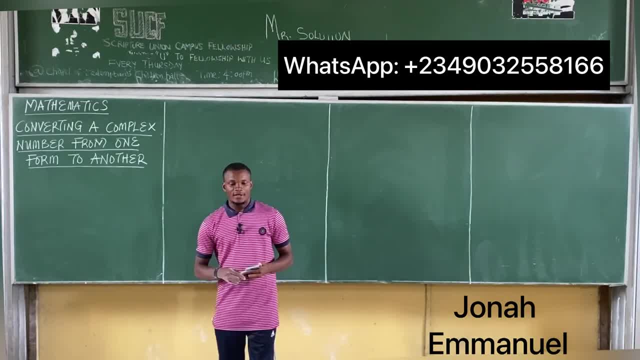 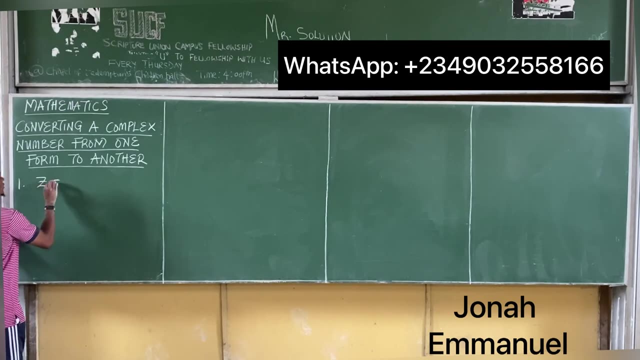 question. Alright, So let's look at the conversion of a complex number from one form to another. Now recall that in our previous lesson we talked about a complex form being expressed in two forms: Z equal to A plus IB or perhaps AB. We said this is the rectangular, or. 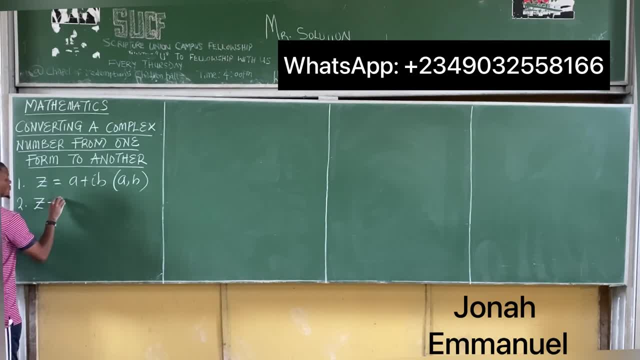 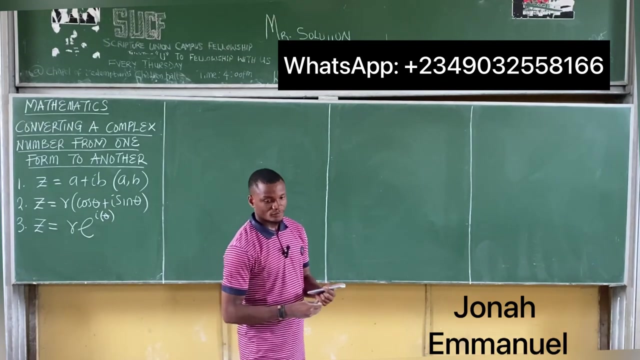 Cartesian form. We talked about Z being equal to R into cos theta plus I sine theta. Recall this the polar or the circular form 3,. we talked about Z being equal to R, exponential I theta, and we call this one the exponential or the Euler's form of. 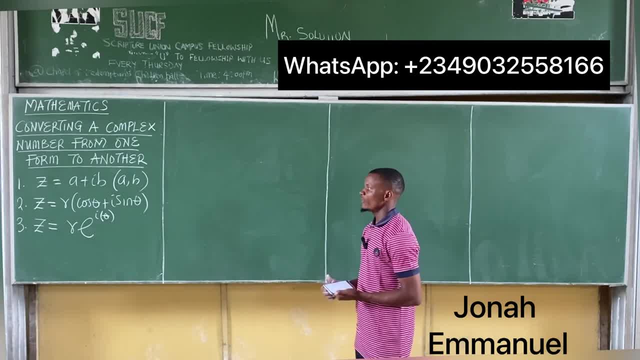 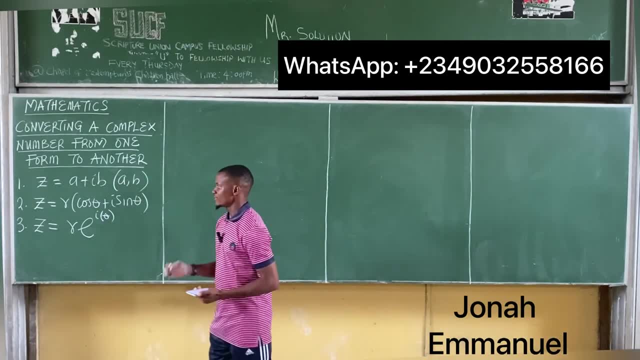 expressing complex numbers. So let's see how we can convert one complex number from one form to the other one. For instance, before you do conversion of a complex number, note the following: Note that R, we said, is the modulus of the complex number. 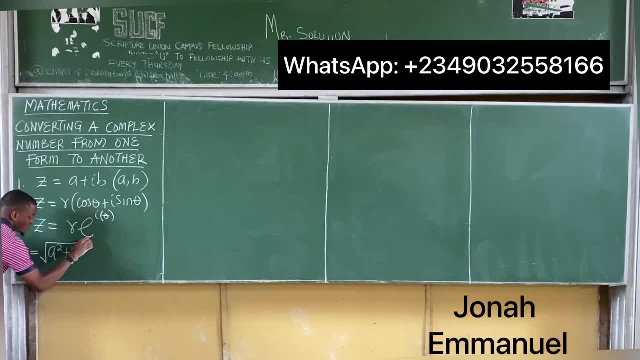 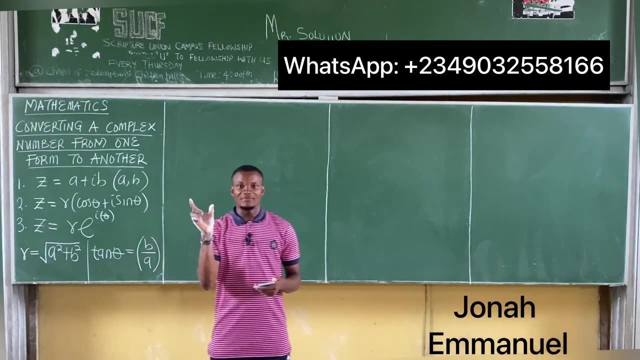 is given by A squared plus B squared. So this is how we get the value of R. Also, note that tan theta is equal to B over A. So we can get theta by taking tan inverse. Tan inverse of B does the imaginary part all over A. That's the real part. 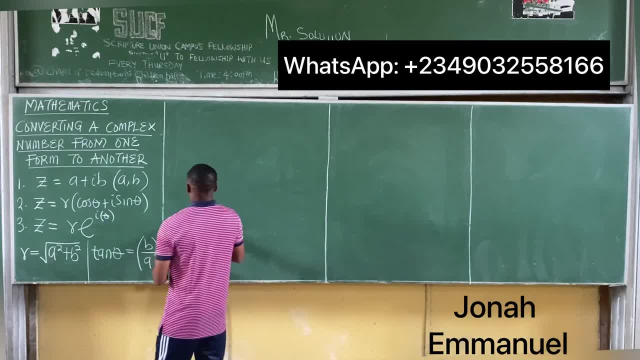 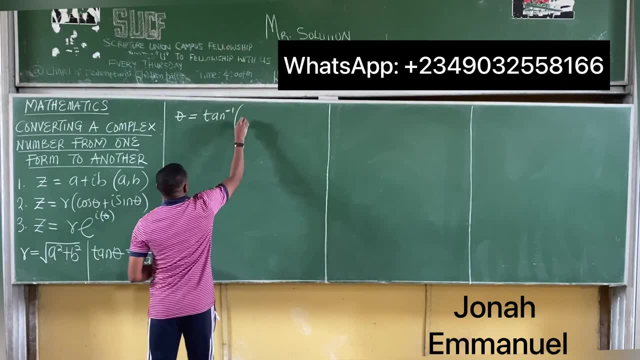 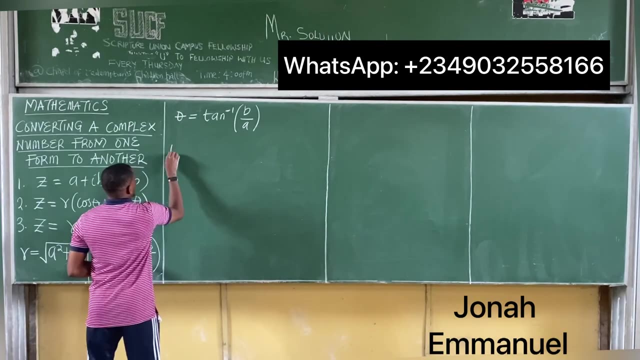 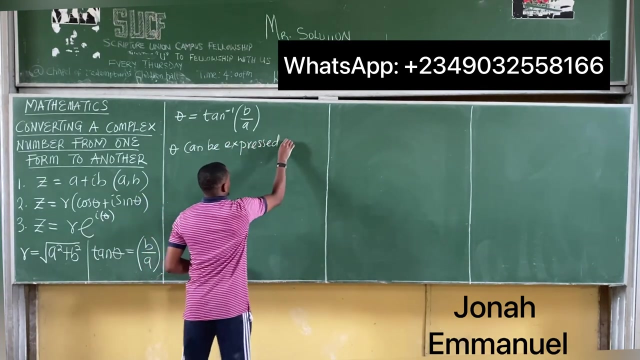 So that's how we get this one here. So it's more like saying theta from here. Theta is equal to tan inverse of B over A. So we have this. One last thing: Note that theta can be expressed in degrees. 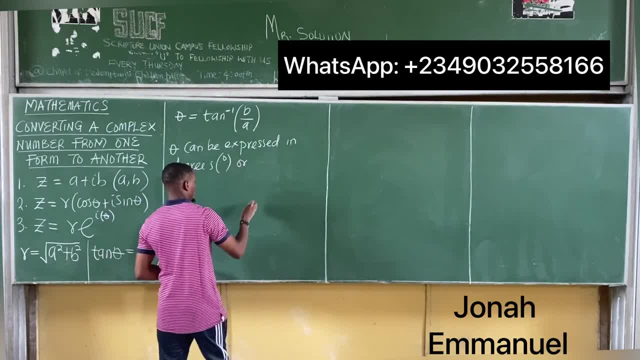 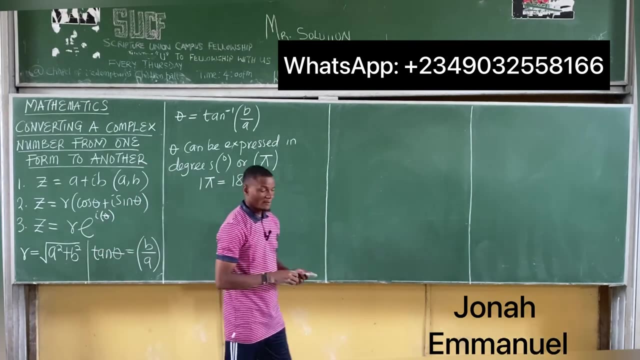 does this or pi Does this All right In degrees of pi, Where one pi is equal to 180 degrees? All right. So we have this All right. So, with this one taken, let's try an example. 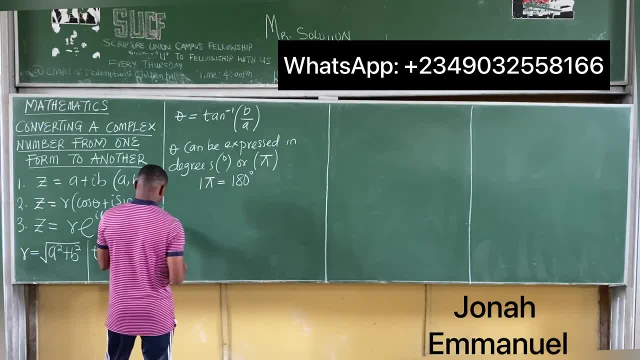 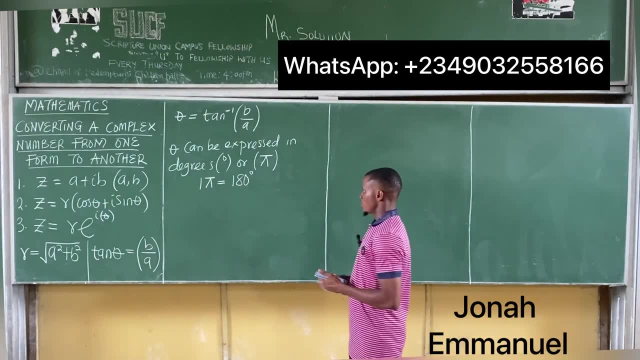 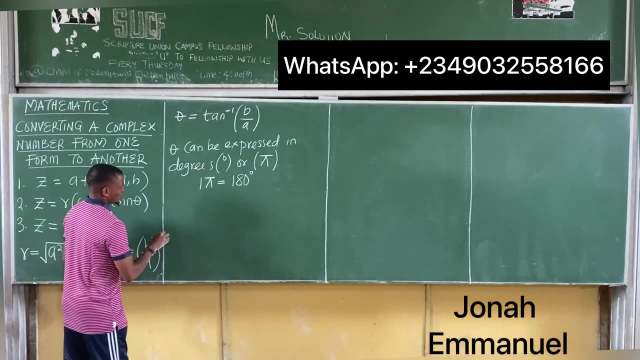 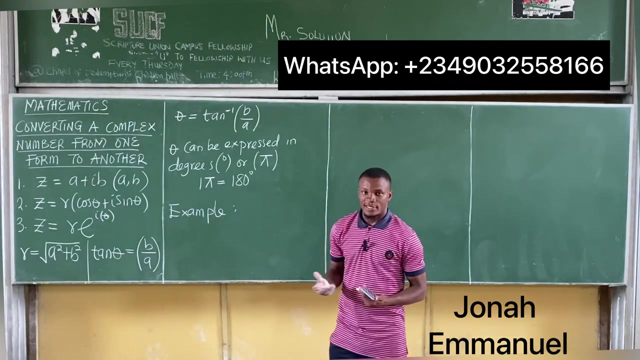 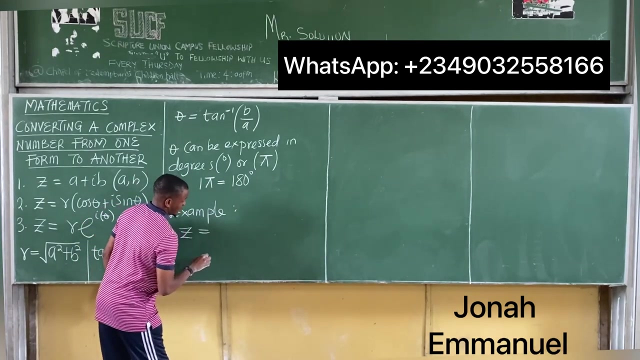 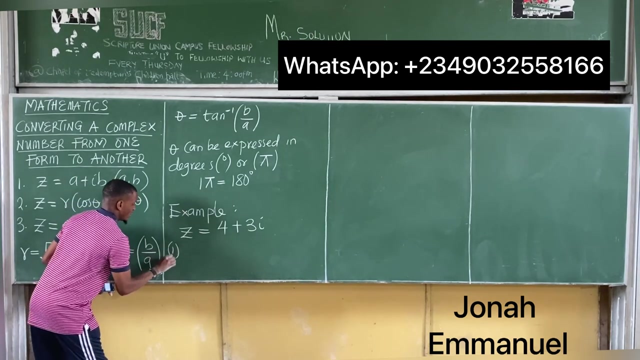 So example, So example. Okay, So if you've gotten this, let's look at an example, For example. let's say we are given, for example, let's say we are given the complex number z, equal to 4 plus 3i. So this is, in rectangular form, number 1. Express this one. 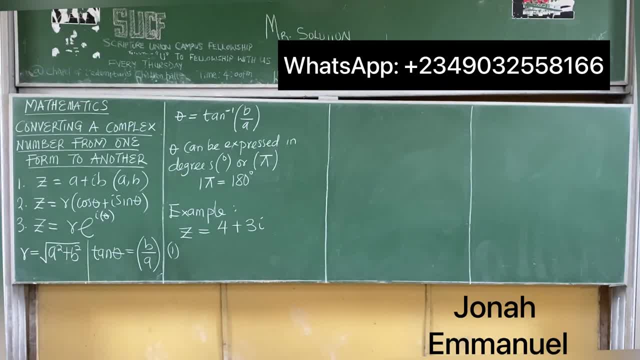 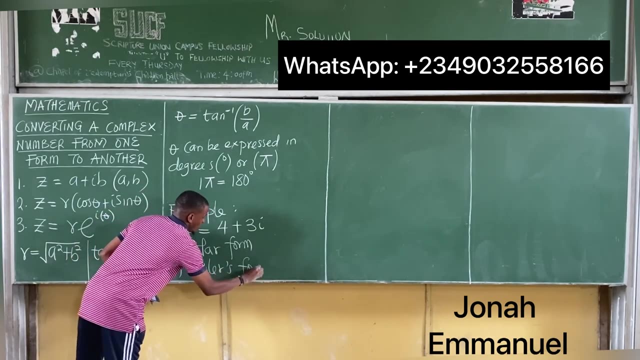 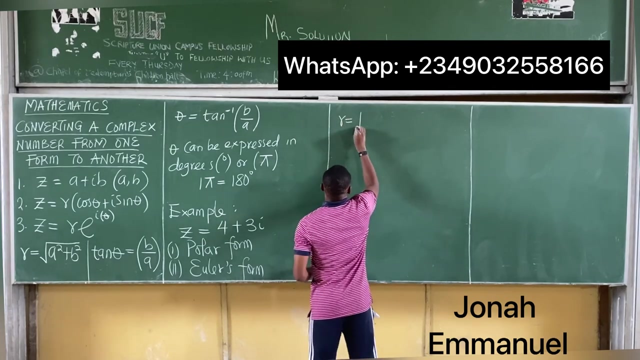 here. And to express this one here in polar form or circular form, Express this one here in Euler, Euler's or exponential form. So first is first, Let's get r. meu Saying r is equal to the square root of this one here. 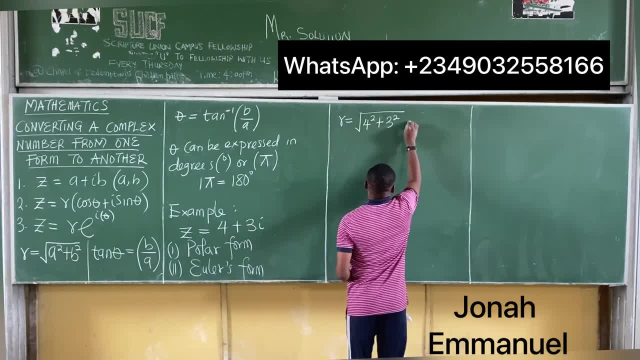 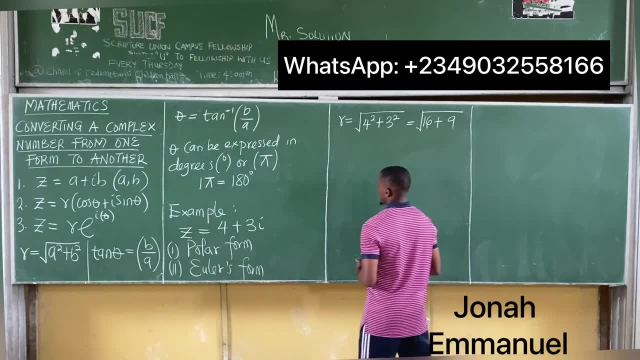 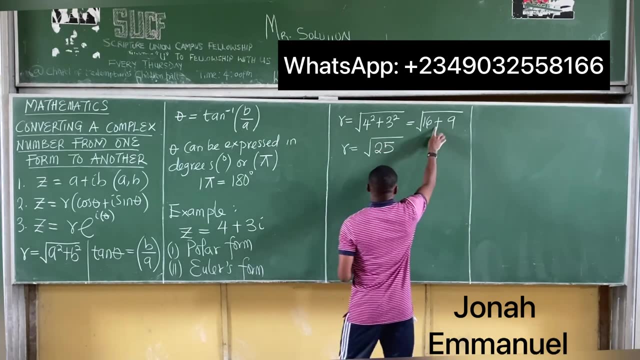 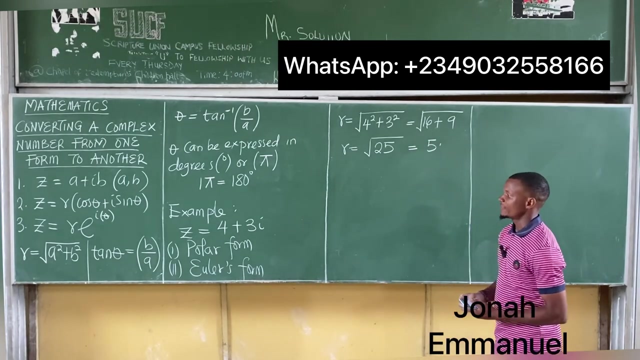 Four squared plus this one here, three square, That's equal to the square root of four square squared is 16 plus 3 squared is 9, so hence r is equal to the square root of these two combined, this is 25, so r is equal to 5. we've gotten the value of the modulus as 5. let's get the angle. 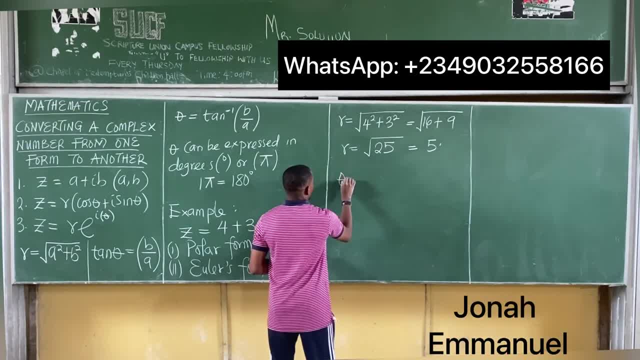 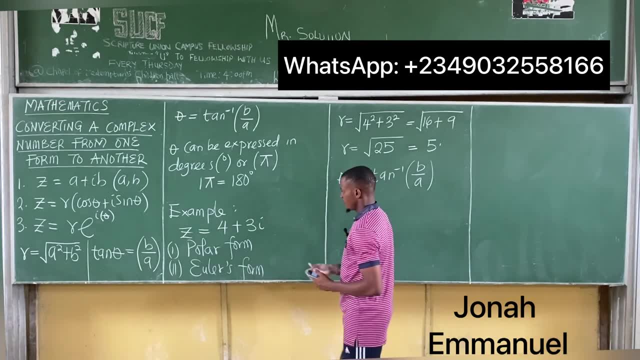 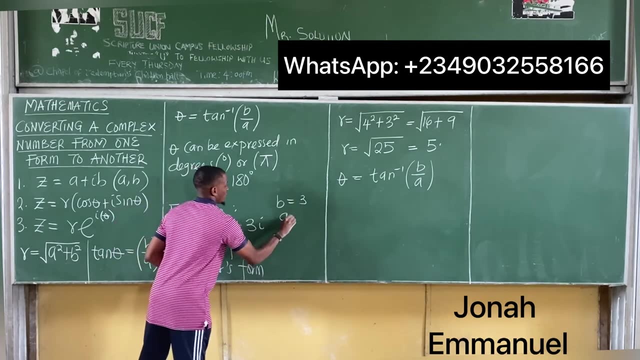 or the amplitude. the amplitude theta, we said, is equal to tan inverse of b over a, given this complex number, here b is equal to 3, that's the coefficient of i here, and a is equal to 4. i have this all right. so this is equal to. 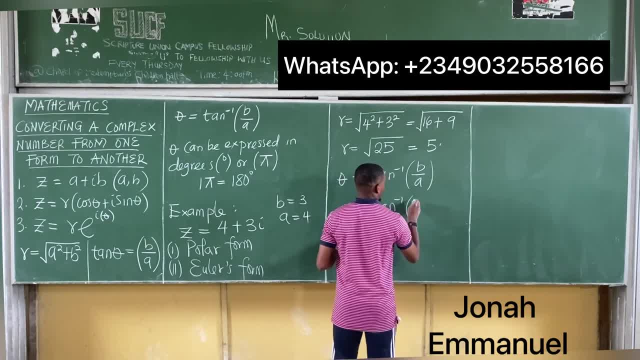 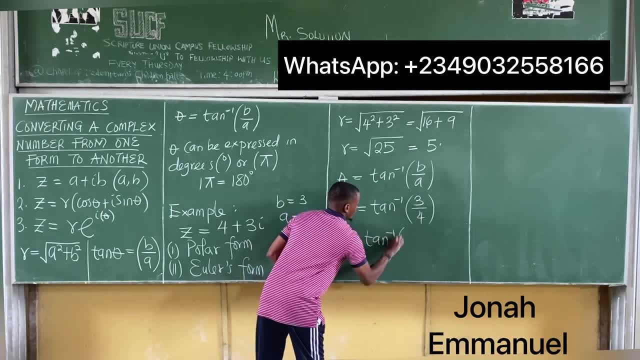 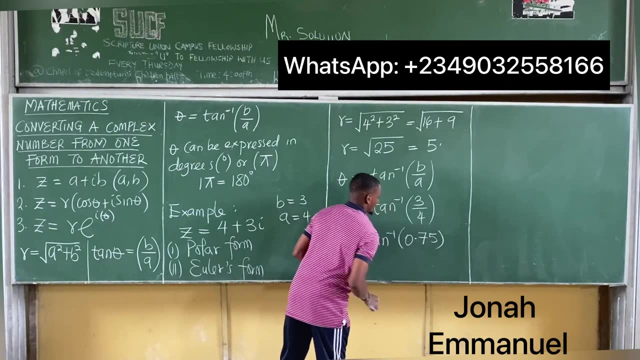 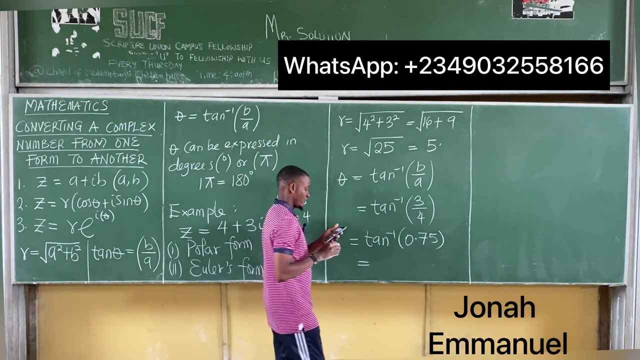 tan inverse of b, that's 3. all over 4, that's equal to tan inverse of 3 over 4, gives you 0.75, 0.. 75, that's equal to tan inverse of 0.75. we have 36.87 degree. so that's theta. so therefore, 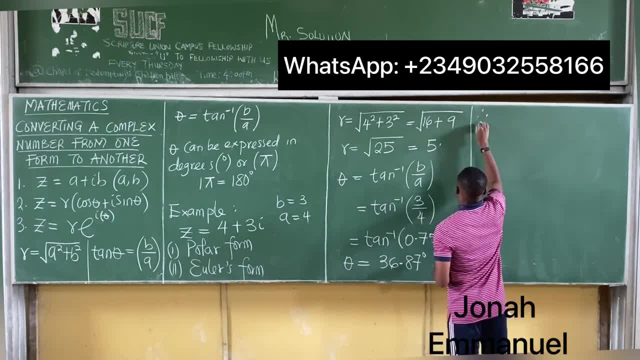 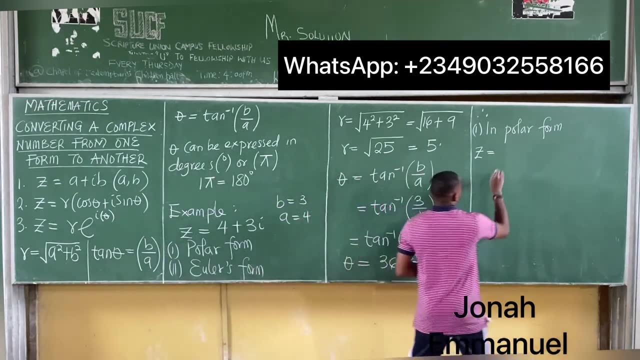 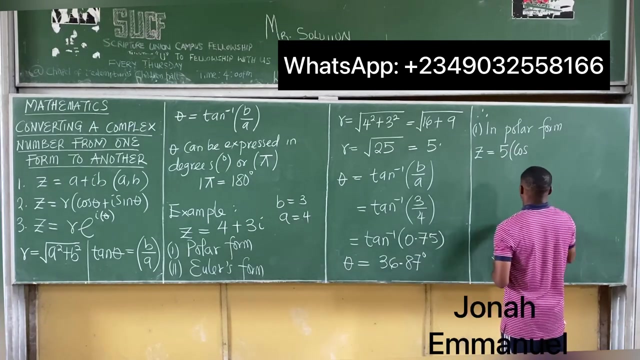 therefore i in polar form. in polar form, z is equal to, we said, r, which is 5. that becomes 5 into cos theta here is 36. perhaps i want to use a round bracket, so i'll change here to a square bracket: cos 36.87. okay, plus i sine theta, there is 36.87. 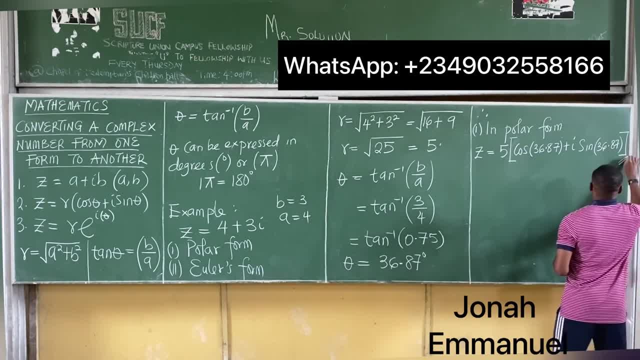 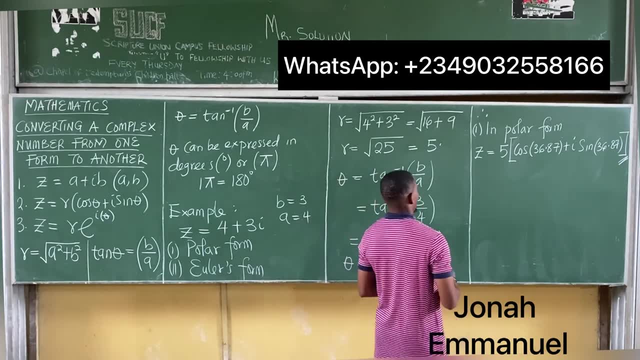 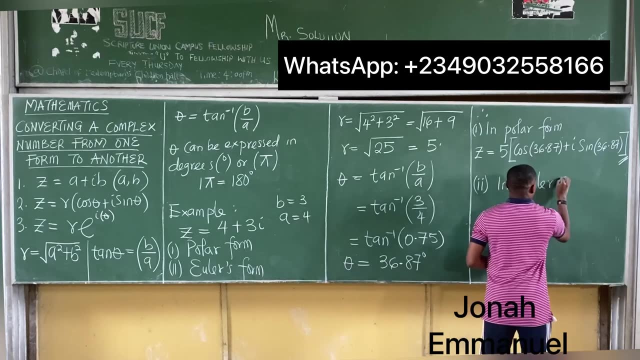 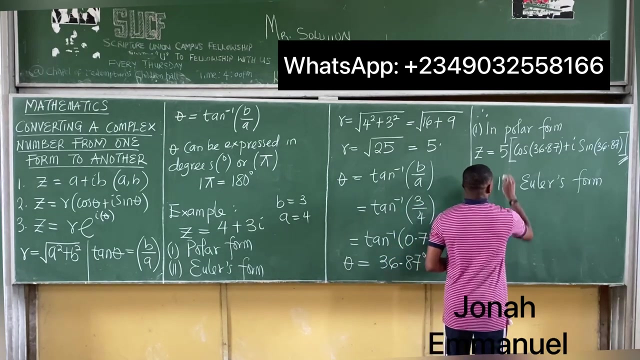 so we have this all right. so this becomes the complex number in polar form. finally, i. i let's get this in euler's form. in euler's form, what do we have? we said in euler's form, z is equal to r, which is 5 exponential i theta. so exponential i theta is equal to r, which is 5 exponential i theta. so 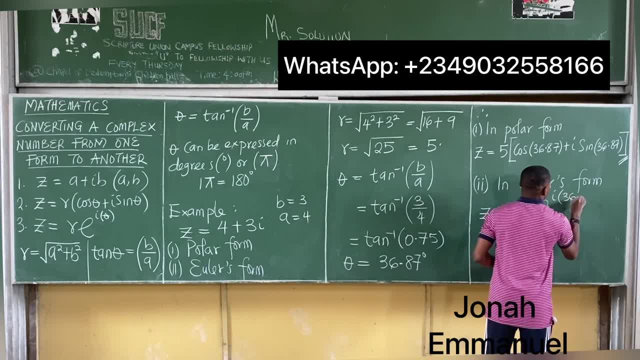 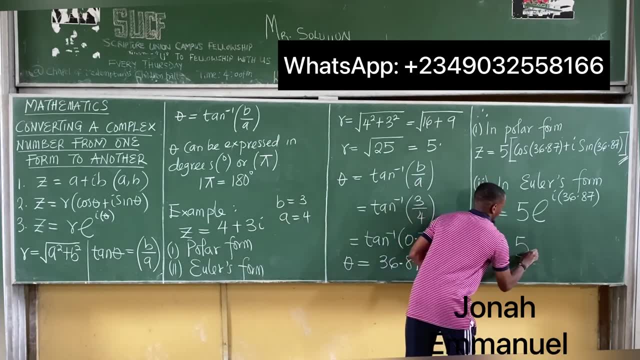 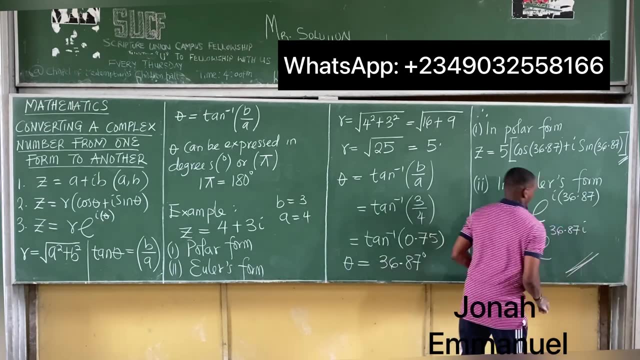 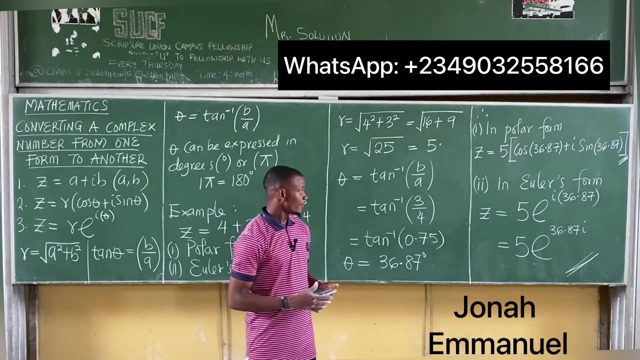 exponential i theta is 36.87, so hence we can leave it this way, or we can say: that's equal to 5 exponential 36.87. i all right, so this is how we solve this. this is how we do the conversion of complex numbers from one form to another. all right so. 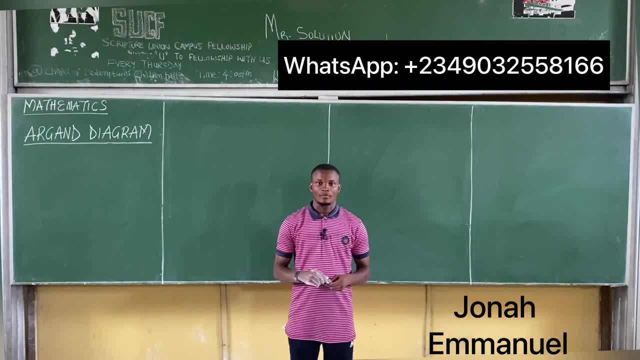 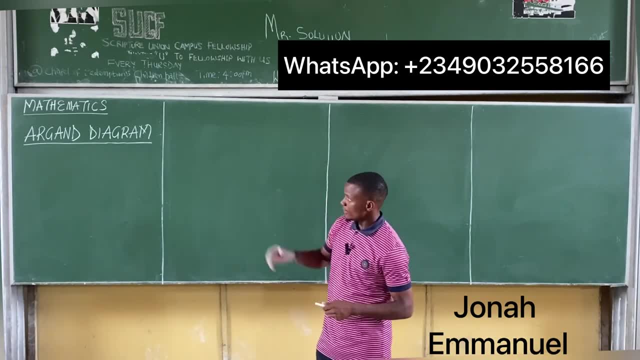 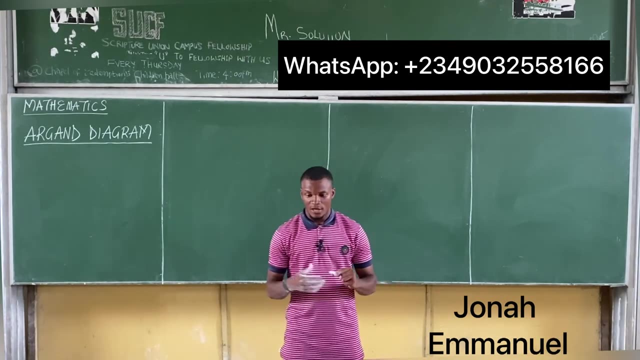 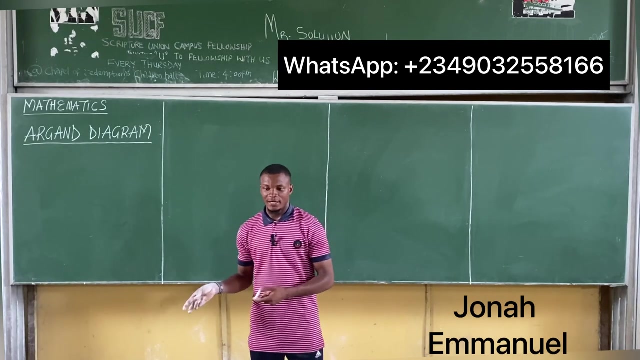 um. look at the next task. hello and welcome to today's class. for today's class we'll be looking at um argand diagram. argand diagram: we've looked at three ways of representing um complex numbers: rectangular, cartesian form, um euler's or exponential form, then polar or 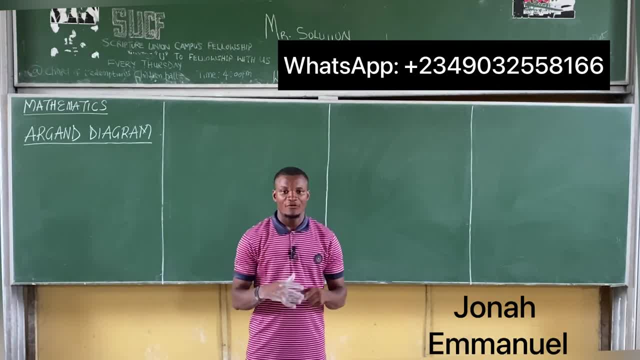 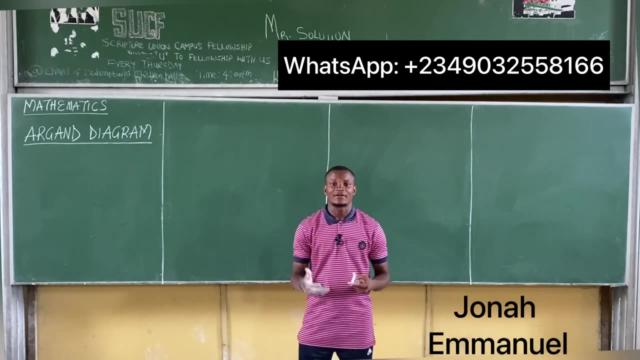 circular form. and the third way is yet another way of representing complex numbers, known as um, using the argand diagram. it's also called the graphical method of representing complex numbers. all right, so what's an argand diagram? an argand diagram is simply a graphical method used to represent 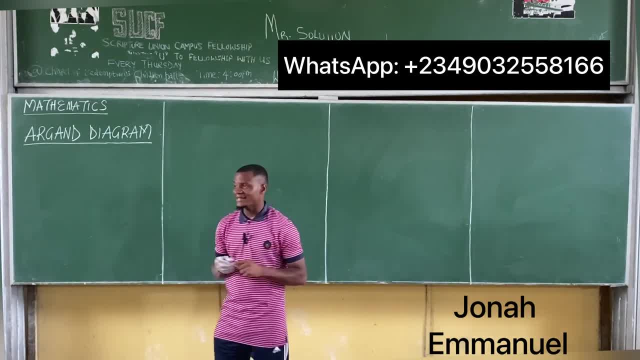 complex numbers. now, how does it work? remember that, when it comes to your rectangular form of complex numbers, you have z ie, z equal to z into t, and z equals 1, z equal to 3, z equals 1, 1, 1, 1, 1, and so this is the difference between the two. well, now, in euler's form, you have 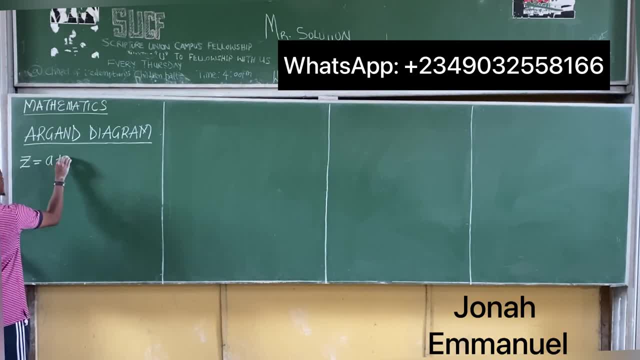 a z and you have a z that are in the square and you have a z that are in the square. so this is the being equal to, let's say, a plus ib, and we said this is the same thing as a and b for this case. here this a becomes your x, y, b becomes, perhaps, your y axis. so don't forget that in a normal 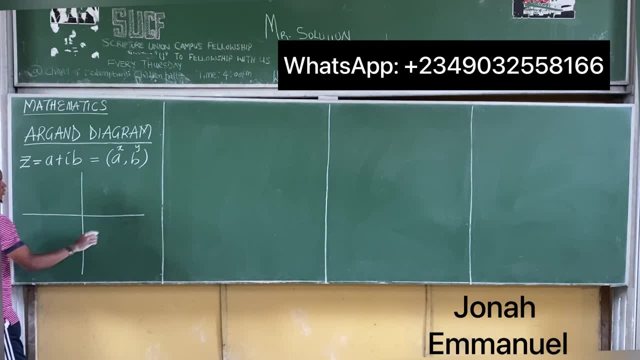 cartesian coordinate such as this. there are four coordinates here- or four quadrants: quadrant one, quadrant two, quadrant three and quadrant four. now for this one here. this axis is called the i axis, so i'm having positive i, no longer y now, but i here becomes the negative i. 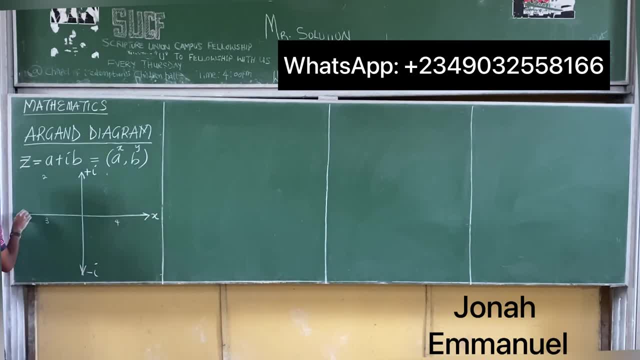 here becomes your x axis, here becomes your negative x axis, because here's a positive x axis and here is negative x axis. so it means if i have a complex number that is positive for x and positive for y, it will be in this region. so this is the region of positive x and positive i value. 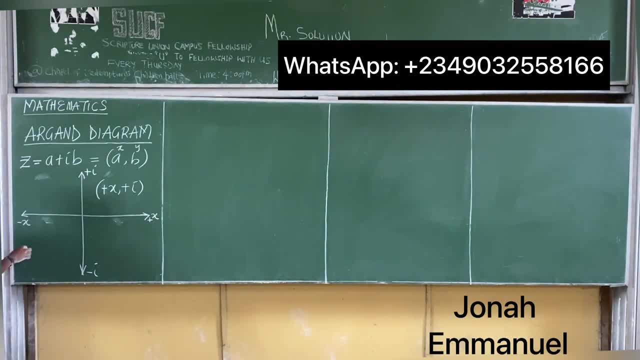 complex number. this region here is for um. this is negative x, so a negative x value or a negative a value and a positive i value will be in this region. this region is for negative x value and negative i value, while this region here is for positive x value and negative i value. i will just 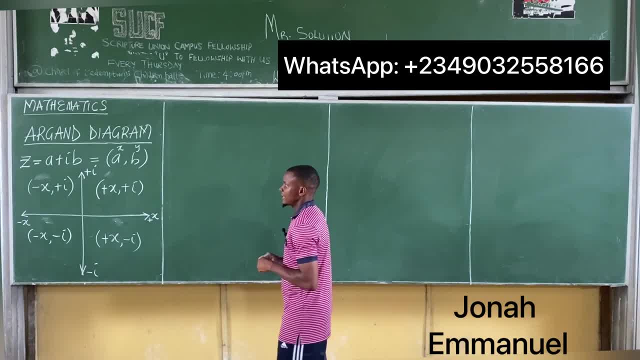 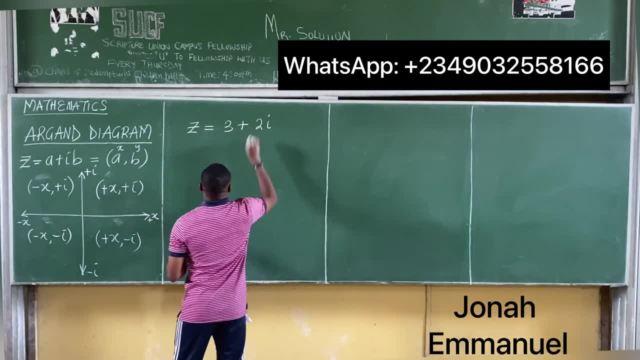 take a few question and we'll see how we plot an argand diagram. let's say i'm giving the complex number z equal to 3 plus, let's say, 2, i. if you observe here the x value is positive and the i value is also positive, positive, positive, that's this side here, positive x. 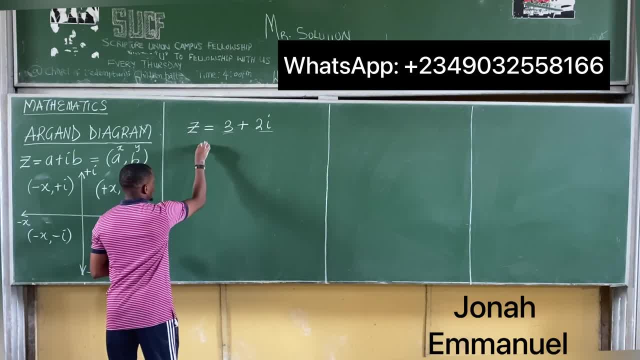 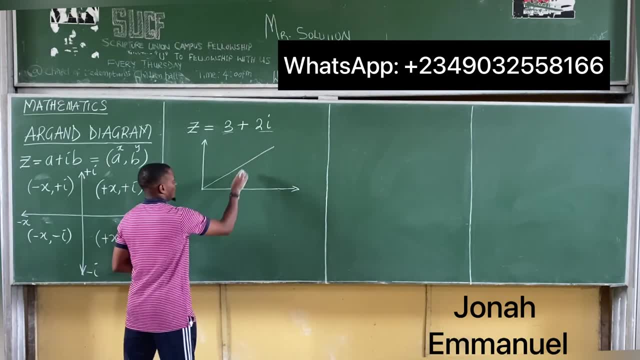 positive i value and negative x value. if you observe here the x value is positive and the i I. so hence my other dagger for this would be something of this nature here, here something like this: for the X is positive, X axis, we said we have three, does a value three? now having three here? so this is three and for you the I is. 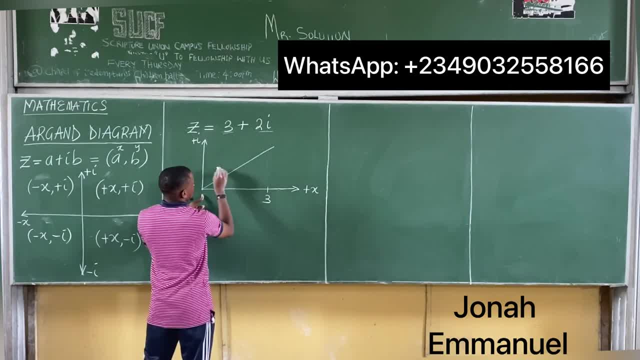 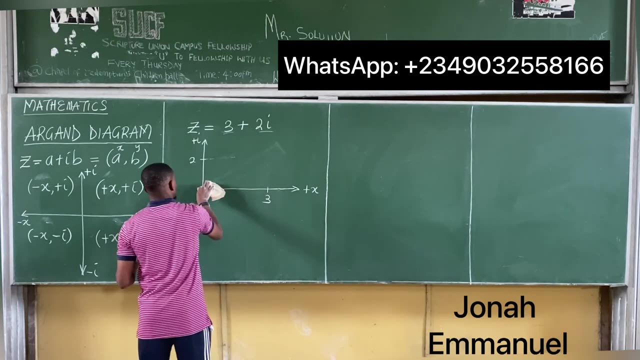 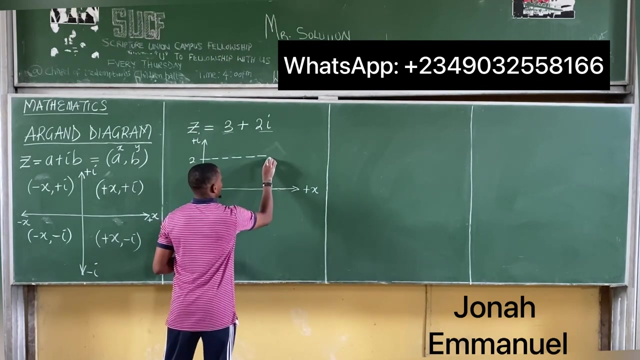 the I region. positive I, of course I have two, so perhaps two somewhere here. two so where the two and the three meets. excuse me, all right, I'm having the positive two here does this and the positive three here does this, so perhaps they meet at this point. so from this point I'll draw a straight line. so this is simply the. 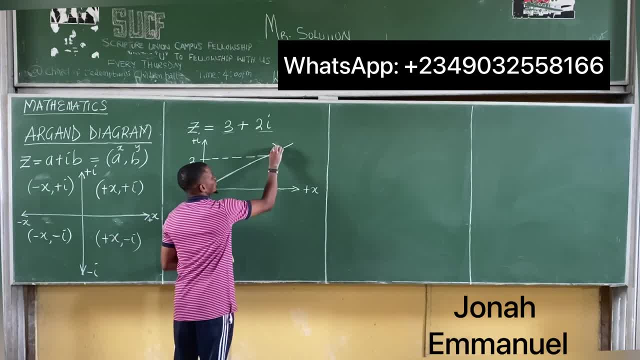 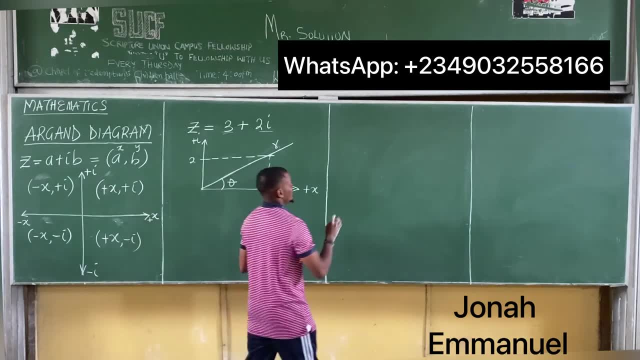 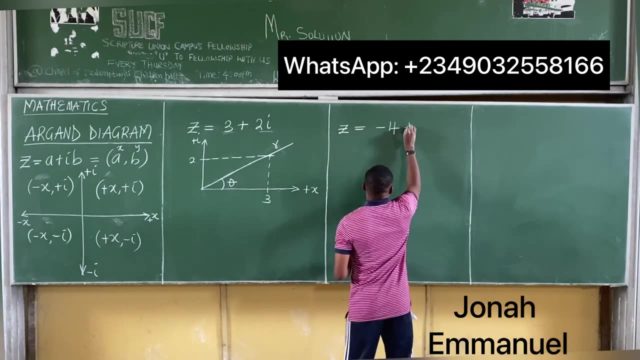 Agand diagram. there are multiple attributes, like the modulus would be here and the amplitude would be here. but this is like the concept of drawing Agand diagram. we'll take one more example. let's say we say, let's say we're given Z is equal to minus four plus three I. but to sketch an Agand diagram, 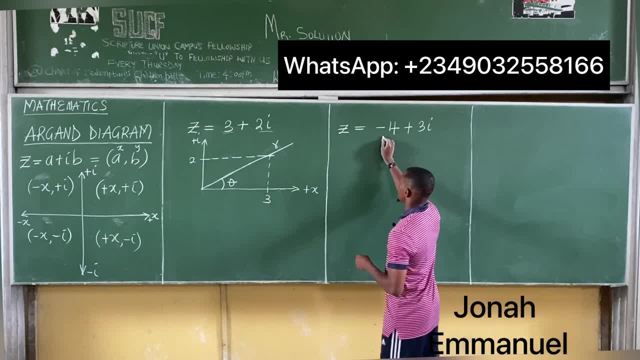 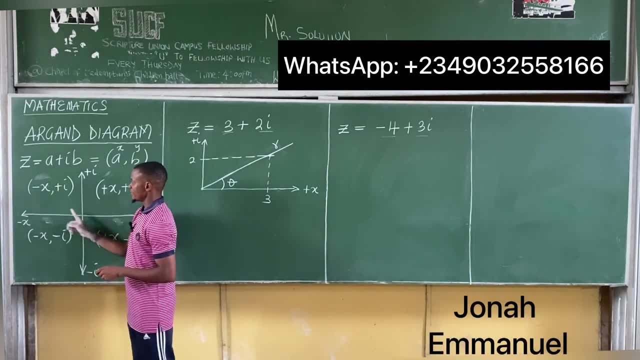 for this. the Agand diagram for this would be: I'm having a negative X value and a positive I, so come back to this. negative X does this way. positive, I does this way. so I'll be drawing quadrant two that looks like this. all right, so I'll be. 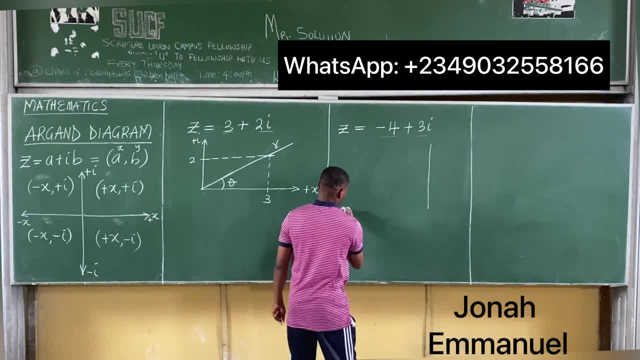 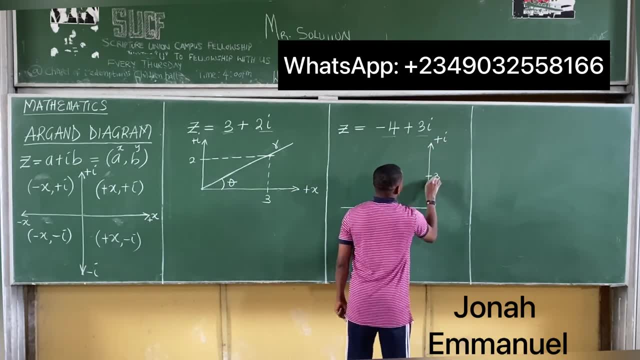 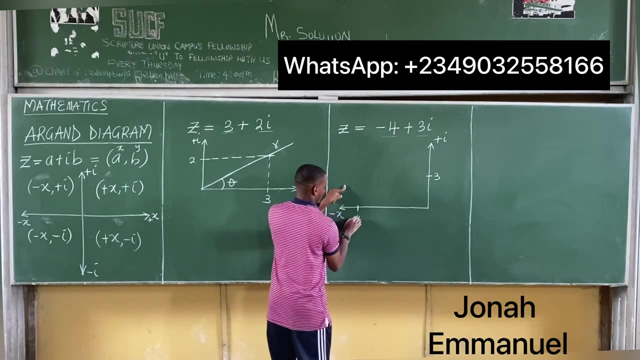 drawing quadrant two here, something of this nature like this, such that we have my positive I value and my three somewhere here, and then your negative X value and perhaps the four. here this becomes a minus four because it's a negative X value. so I'm having this, okay, and then this one here, and then this one here. 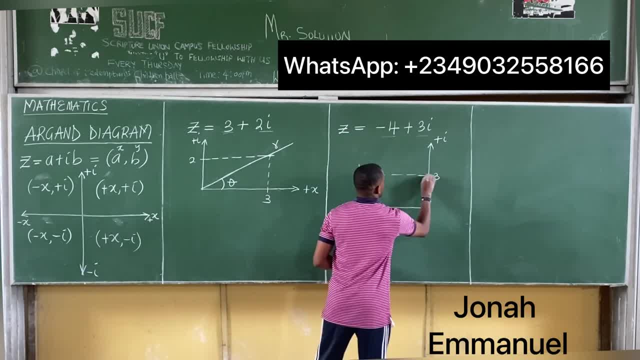 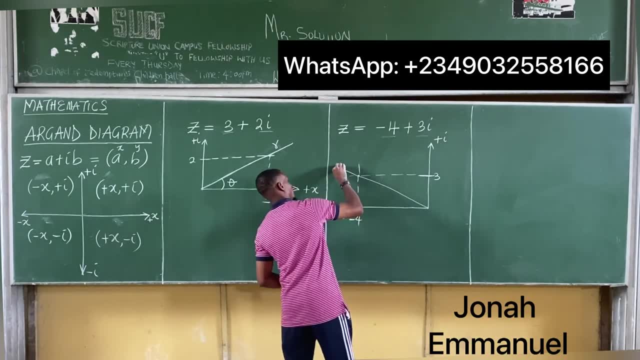 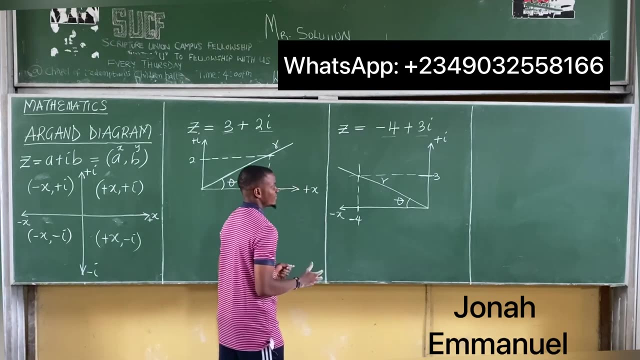 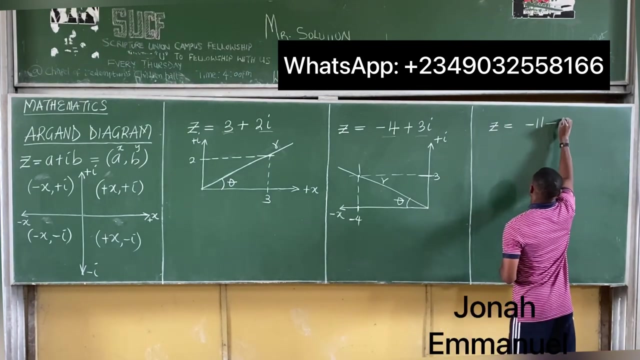 all right, so please, this is a board sketch. we'll meet somewhere. let's say, here now, now draw this this way. all right, so this becomes the value of the amplitude. your modulus will be here. so this is the Agand diagram format. one last thing there. let's say I'm given Z as equal to minus eleven minus I, for. 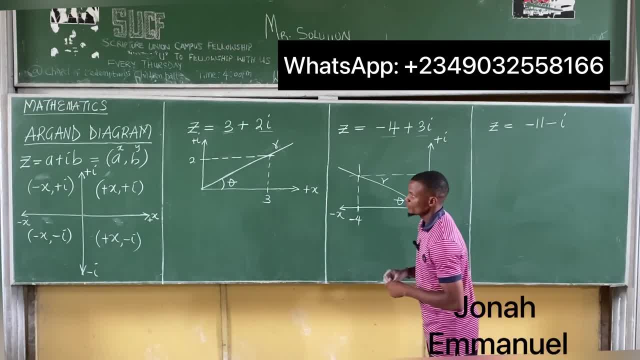 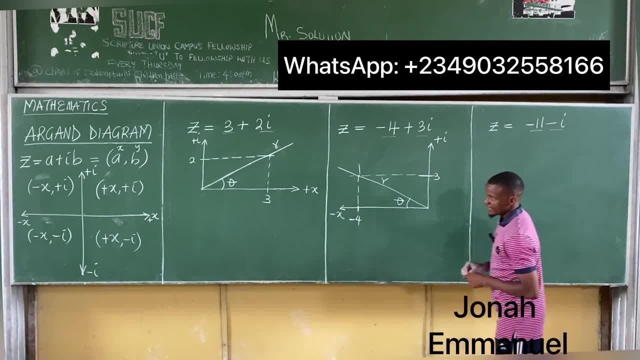 instance, and I want to do the Agand diagram sketch. what do I do? if I look at this? this is a negative of X and negative of I. negative X, negative I. this is the quadrant, this one here, so you can see the motion, the way of. 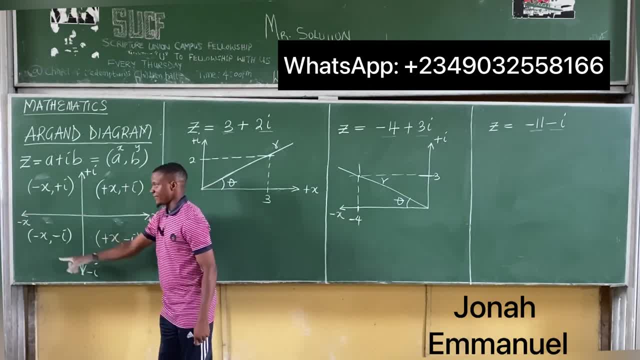 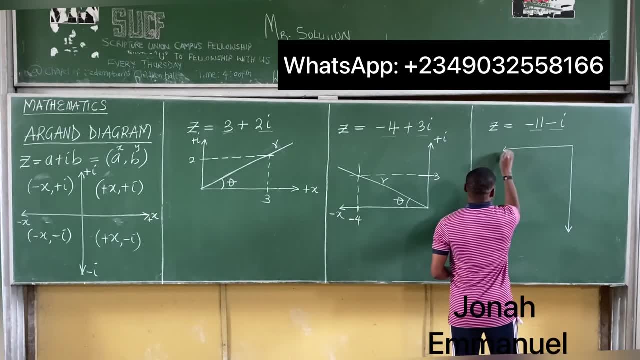 drawing this like this and like this: negative X, negative I. so I'll come here, I'll draw this this way and then this way. so I'm having this here: this is negative X, this is negative I region negative X. we said you're having here as minus 11 negative I. we have in here as minus 1, so if we draw them together we'll 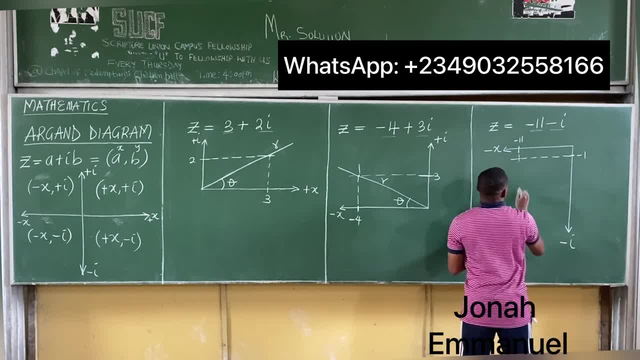 be having something that looks like this. so from here, try to join them. we're having something of this nature. sorry, this line is bent. let me draw a better line. so minus 11 and minus 1, so we'll have something that looks like this: theta would be this and R would be this. so this is what the Agand diagram. 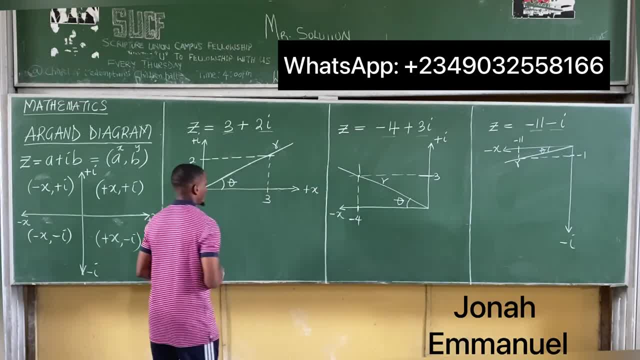 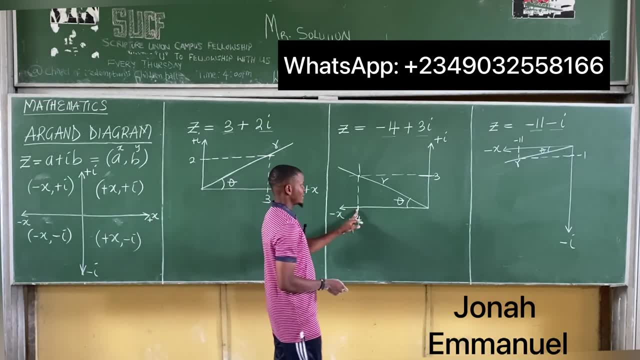 would look like. please notice that for an Agand diagram, let's take an Agand diagram. for an Agand diagram, note that you need the values of the X and the I. you also need a value of the amplitude, theta, and then the modulus R, then you 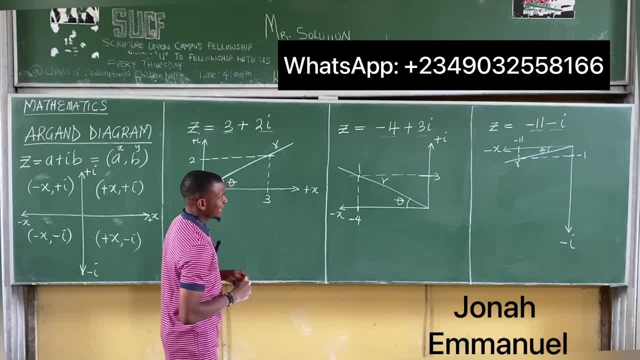 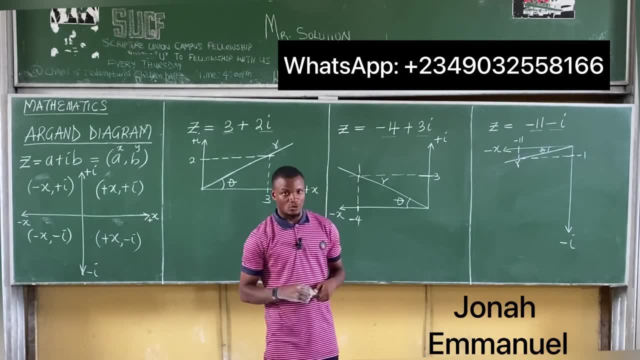 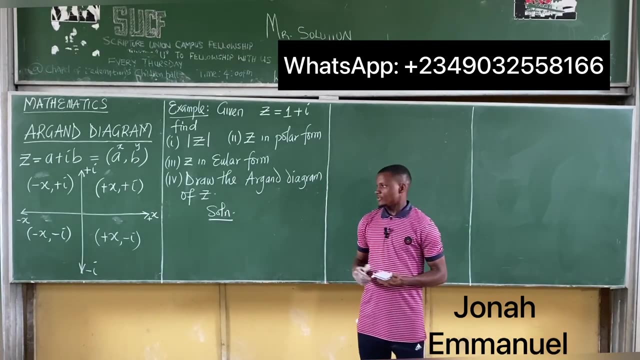 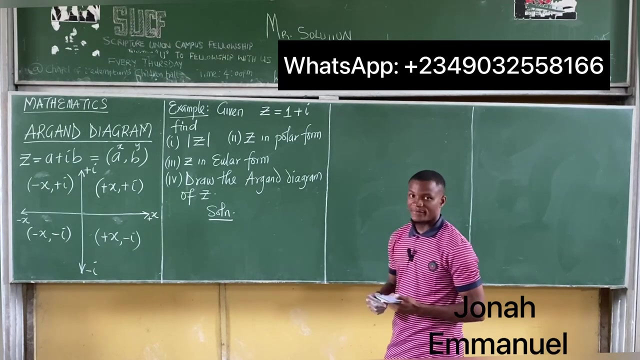 can now guess the full form of the Agand diagram. so this is how an Agand diagram works. we'll take a question and try to draw the Agand diagram. all right, so let's look at this question on the Agand diagram. it says: given that Z is equal to 1 plus, I find number 1. you have that. that means the. 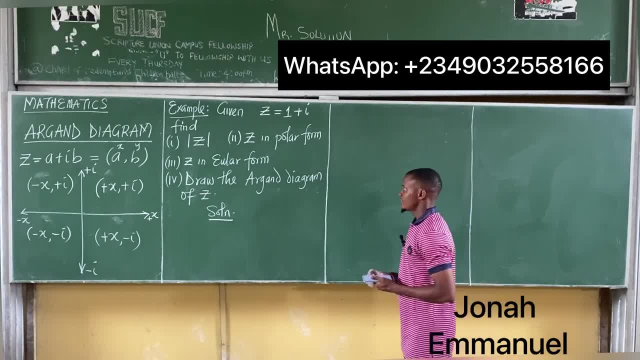 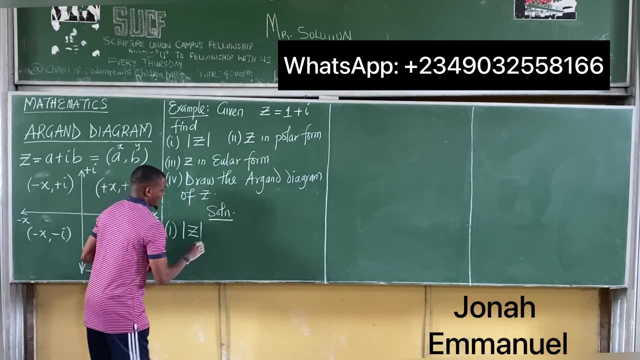 modulus or magnitude of Z. II said it says: find Z in polar form. III: find Z in Euler's form. IV: draw the Agand diagram of Z. alright, so what do we know? number one: we knew that this one here means magnitude. I said magnitude is same as R, which is equal to the square root of the. 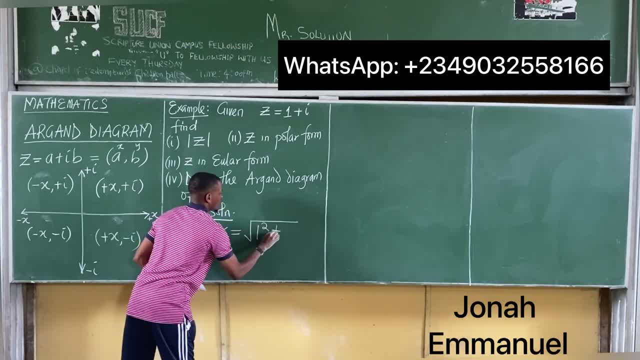 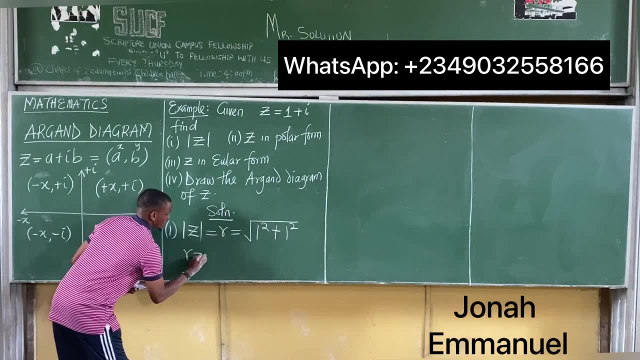 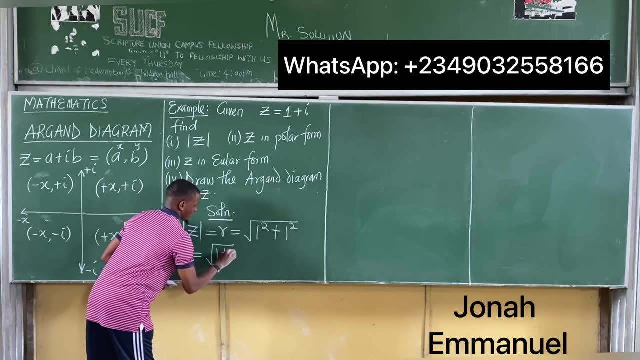 coefficient here is 1, so it becomes 1 squared plus the coefficient here is 1, that's 1 squared. so this is how we get magnitude. so hence R is equal to the square root of 1 squared is one plus 1 squared is 1, that's equal to root 2. 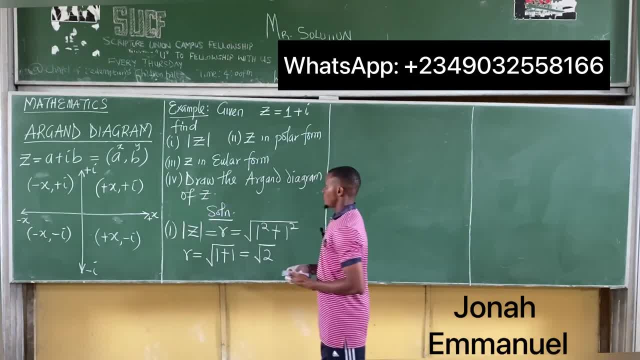 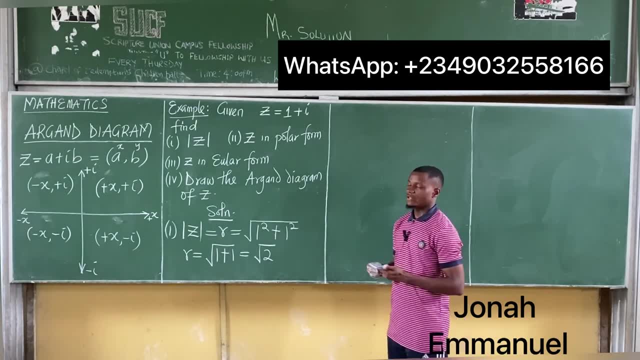 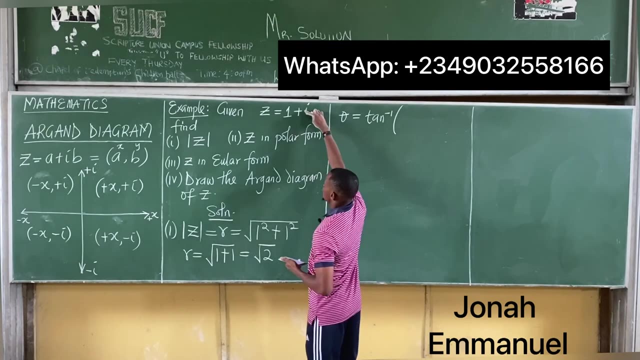 so here's the value of r. next we have to find z in polar form. to get the value of z in polar form we need what's it called the amplitude, and we said amplitude theta is equal to tan inverse of the coefficient of i here, which is 1. 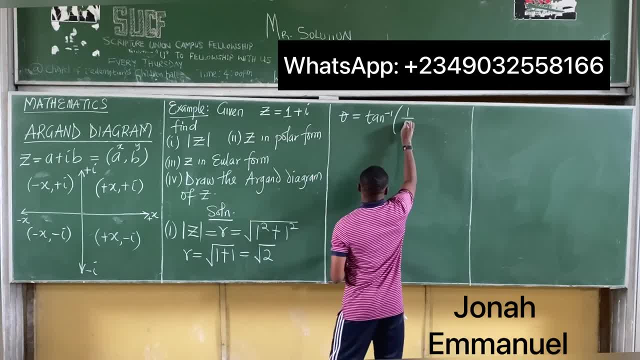 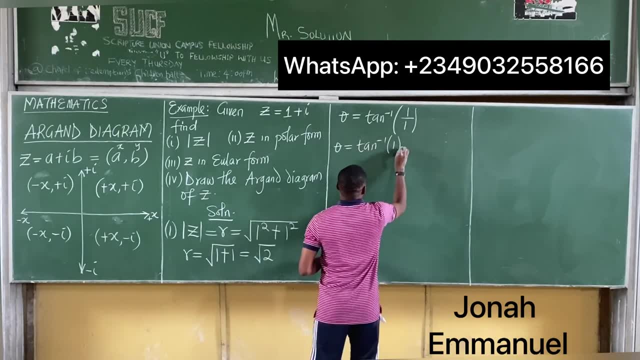 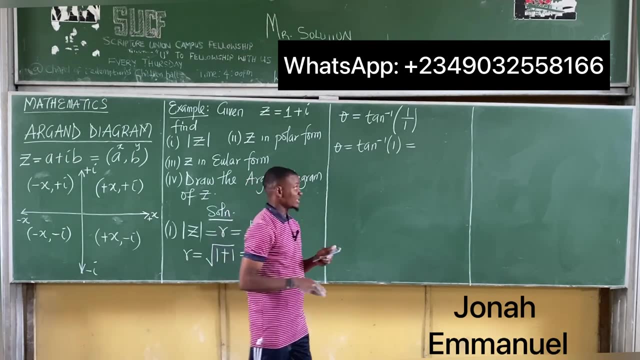 all over the real part here, which is 1, so theta is equal to tan inverse of 1 over 1 is 1, hence theta is equal to tan inverse of 1. that's about 45,, 45 degrees. remember that we said we can express theta in terms of degrees or in terms of phi. 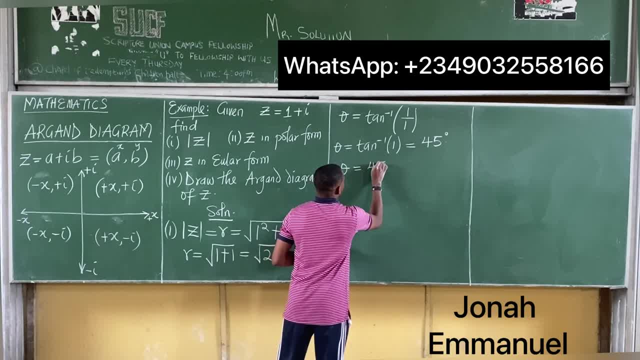 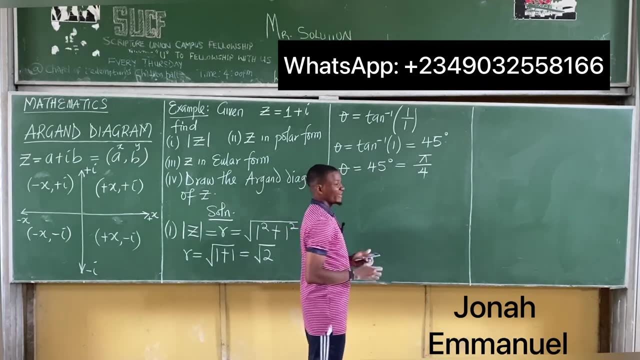 so theta is equal to 45. degrees is equal to in pi. we said pi is 180, so in terms of pi it becomes pi all over 4, the idea is that 180 divided by 4 gives you 45, that's it. 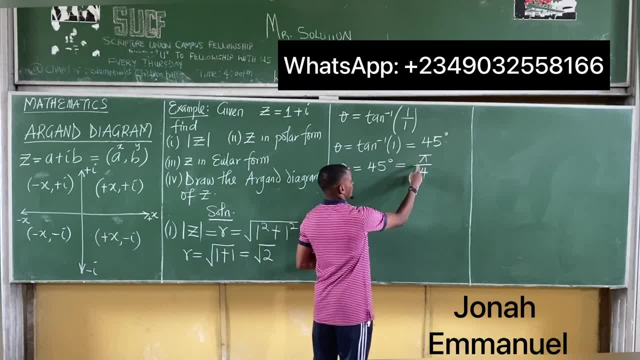 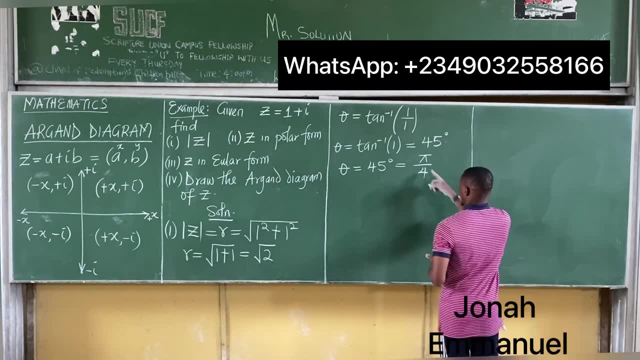 so 180,. pi is 180, so 180 over 4 gives you 45, that's how we express this one here in terms of pi. to get the pi value. this is what you do. you just come here, you just say: 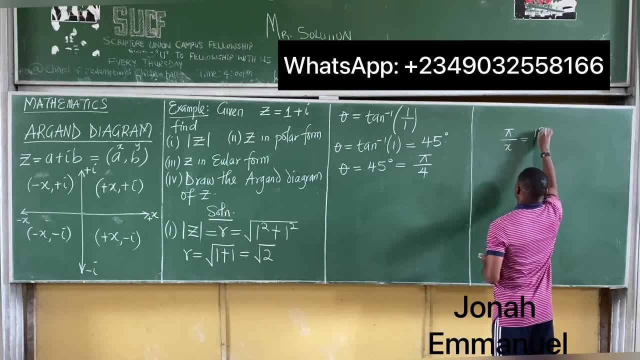 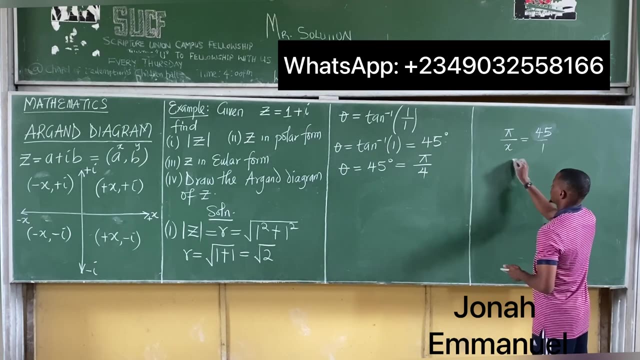 pi all over x equal to equal to theta value, that's 45. alright, just take this one as x. pi over x is equal to 45 degrees. if you cross, multiply pi times 1,. pi equal to 45 times x is 45x, but we said pi is 180. 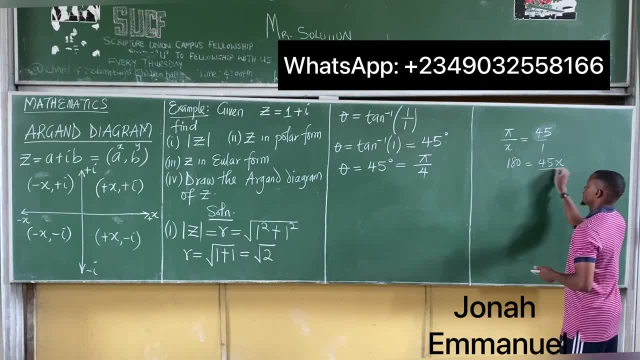 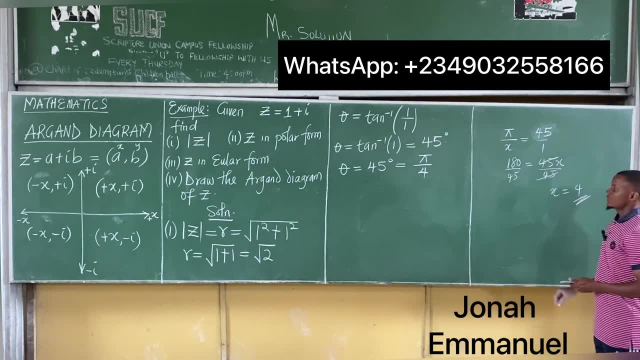 so change here to 180 divided by 45,. divided by 45, this will cancel this. x is equal to 4, that's how you can easily get that. so it becomes 180 over 4 gives you 45. this is how to get the 4, alright, pi over an unknown number. 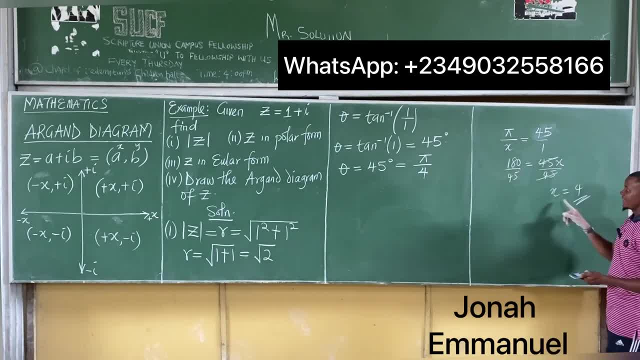 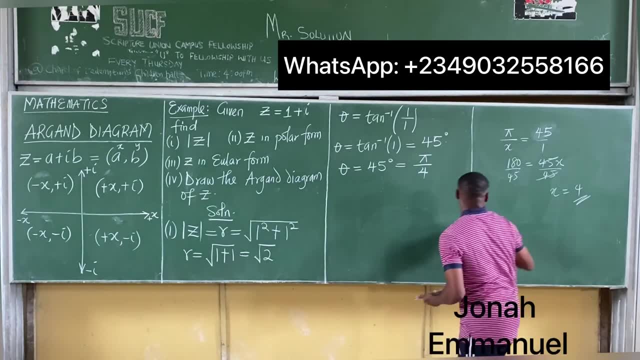 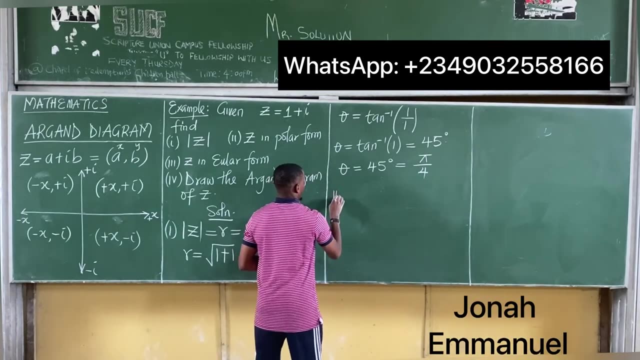 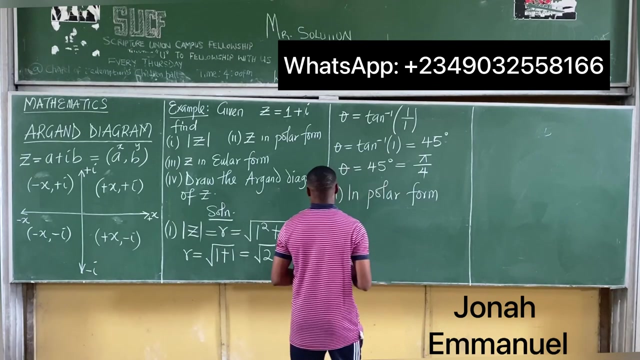 is equal to the gotten angle. cross, multiply and find x. our value here is 4, so therefore, so therefore, ii, ii in plural form. therefore, in plural form, we have that z we said. in polar form, z is equal to r into cos theta. 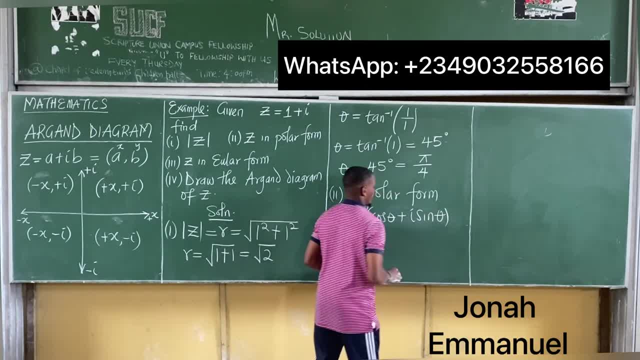 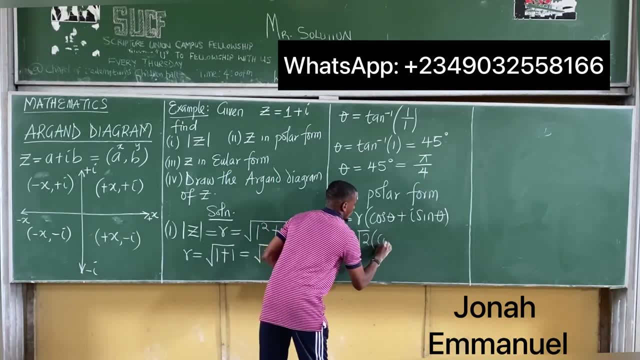 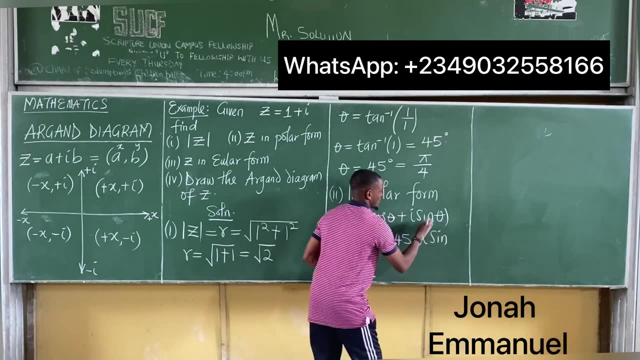 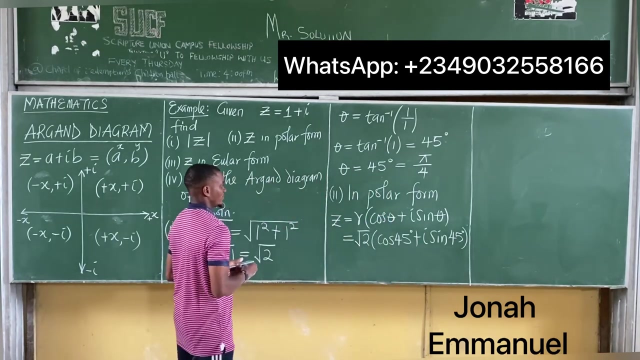 plus i sin theta, that means z is equal to r, r is root 2. so root 2 into cos theta is 45 plus I sine theta is 45 degrees. So I have this Alright. so this is the value in polar form. We can still. 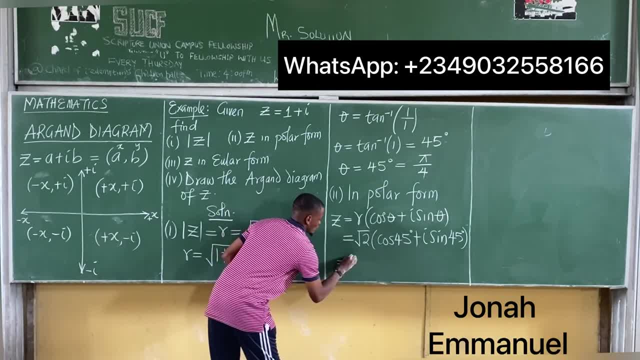 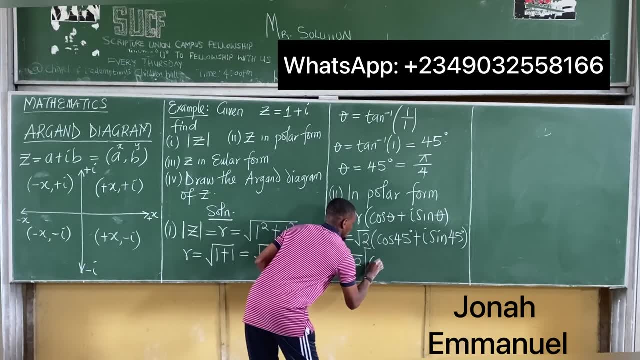 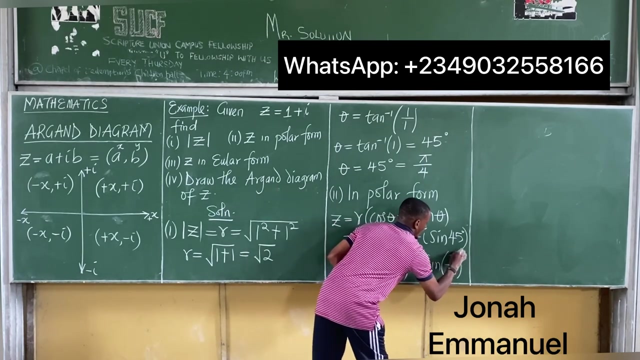 work with pi. In terms of pi, that's equal to root 2 into. I'm having cos, so it becomes cos. 45 inside is pi over 4, pi over 4 plus I sine. 45 inside is pi over 4.. This still works. So this is the polar form. 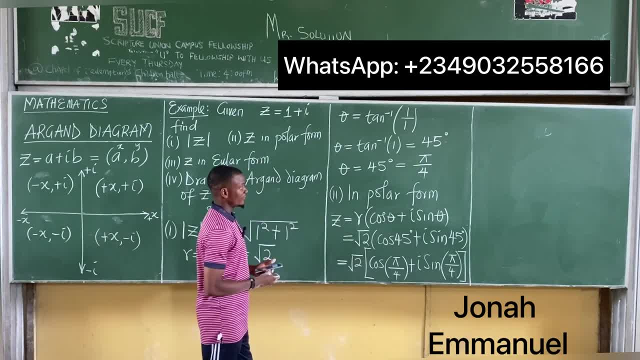 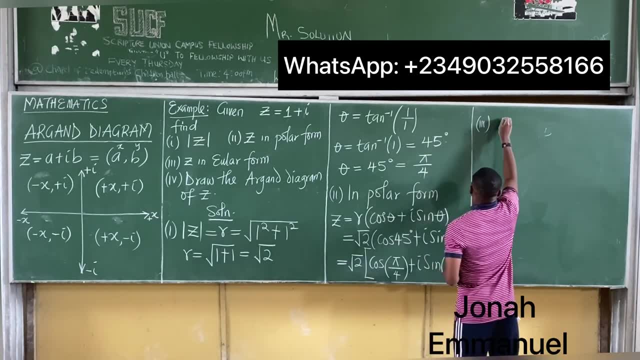 in terms of degrees, This is the polar form. in terms of pi, I, I. I says in Euler's form: I I I in Euler's form. in Euler's form, don't forget, we said in Euler's form, z is equal to. 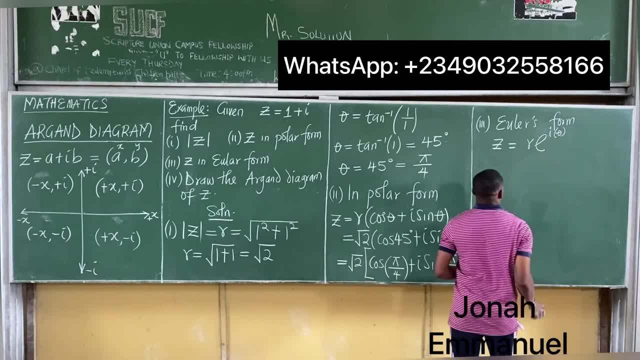 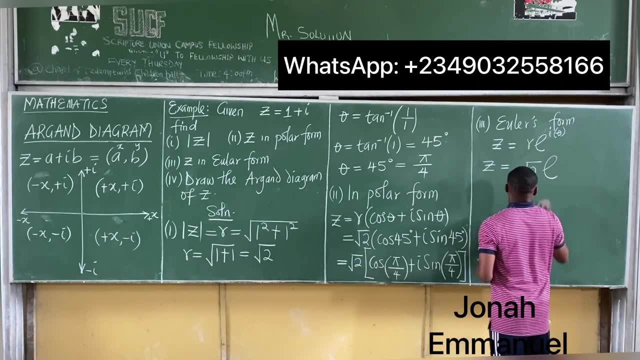 r exponential i times theta. So hence, in Euler's form, z is equal to r. that is root 2 exponential. that's equal to. r is equal to root 2 exponential i times theta is 45 degrees, So that's equal to. 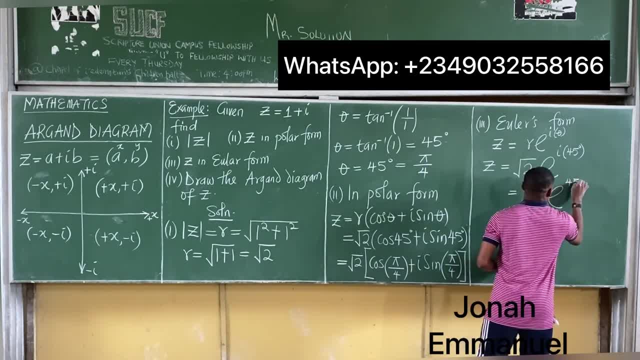 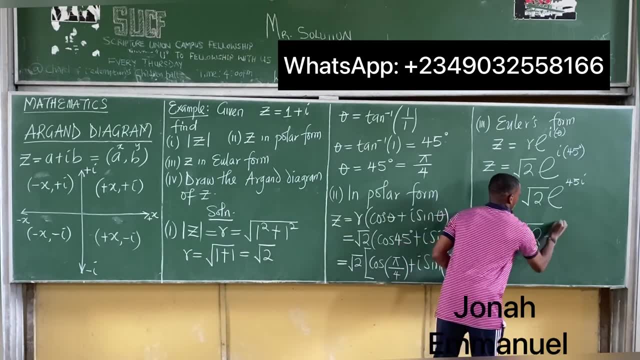 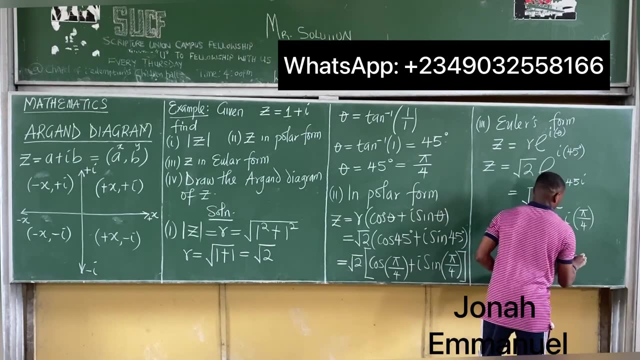 root 2 exponential 45 i. This works. Or in terms of pi that becomes root 2 exponential i. pi is 45, is pi over 4. also works, all right. so this is how we express this in Euler's form. one last: 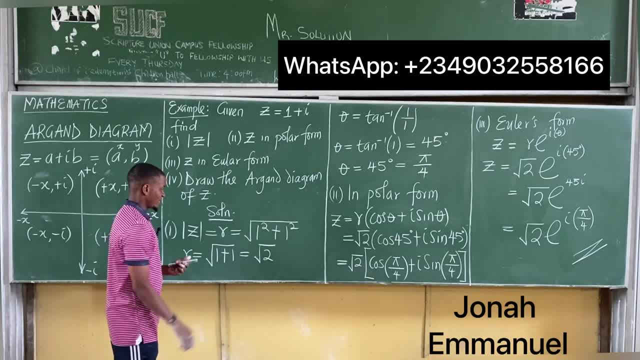 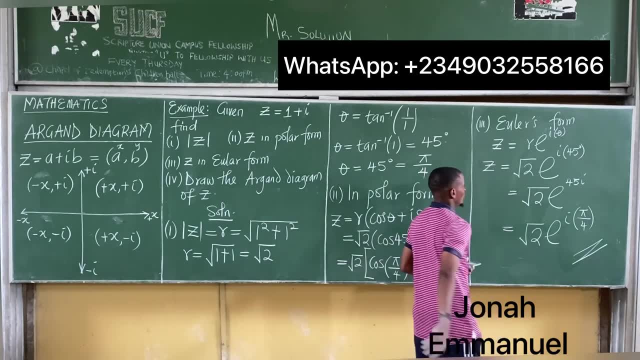 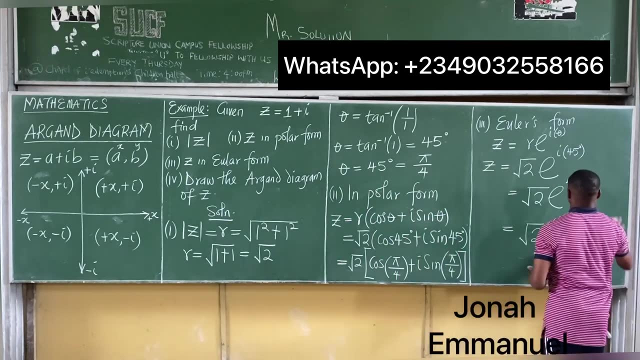 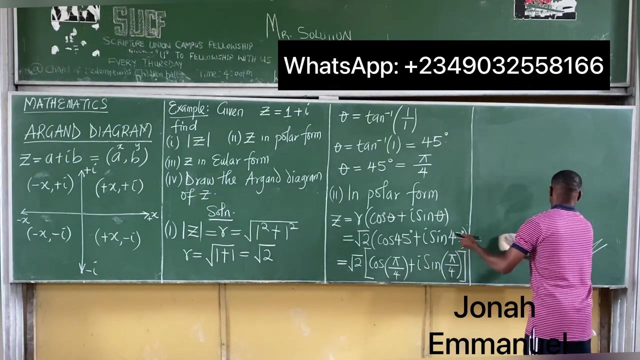 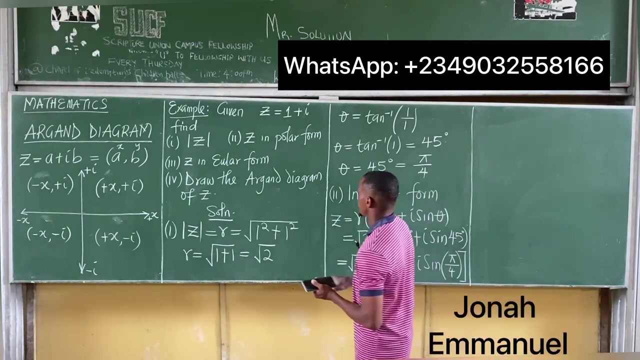 one. we have to find or draw the argand diagram. so let's get the argand diagram. I'll simply take this one off and draw the argand diagram here and that'll be it. all. right, let's get argand diagram for this. so if I look at this question here, 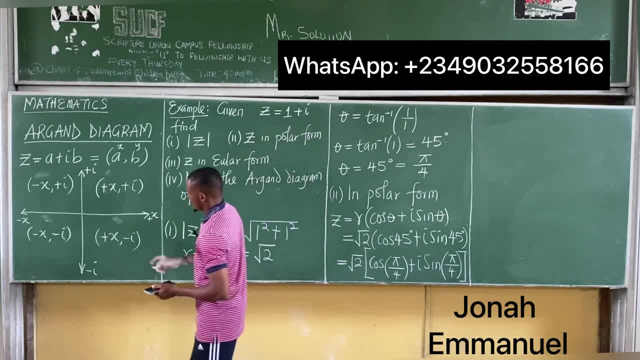 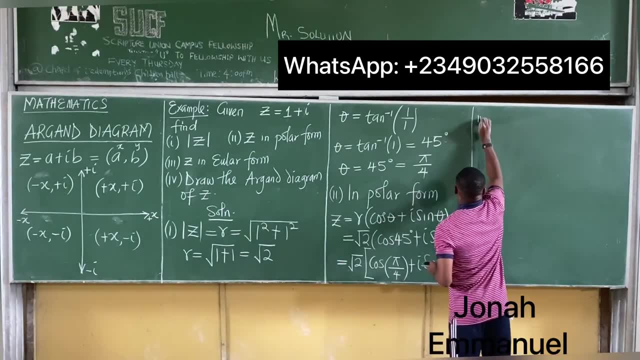 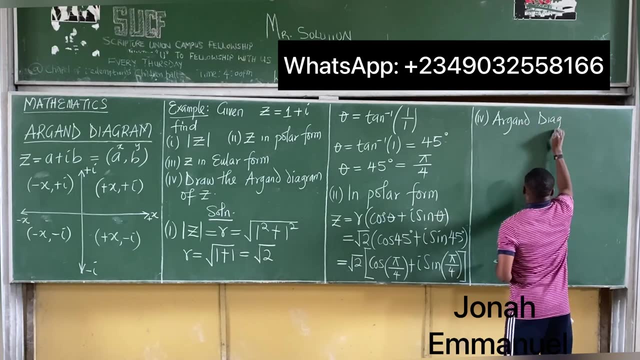 this is positive, this is positive, positive, positive. this is my. I'm using quadrant one of the argand diagram so it becomes quadrant one. so IV4, the argand diagram, argand diagram. I have this one here and then this one here, so this is my positive I. this is positive. X and the. 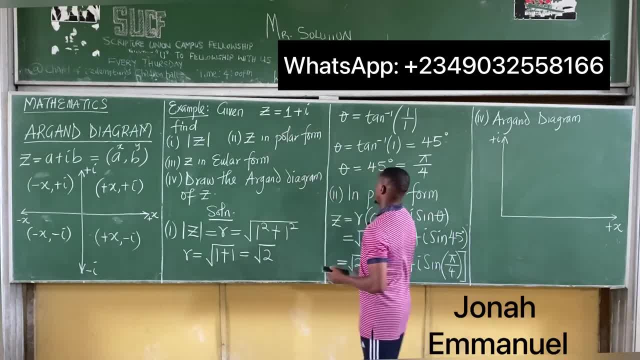 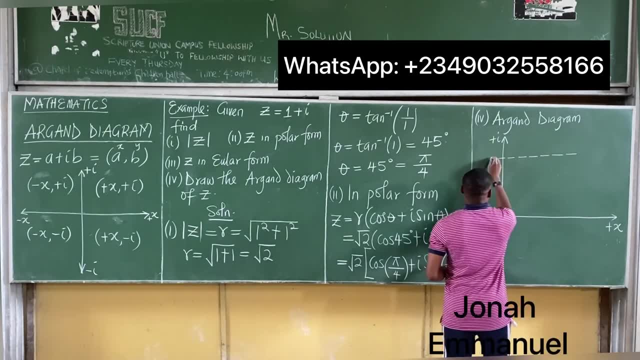 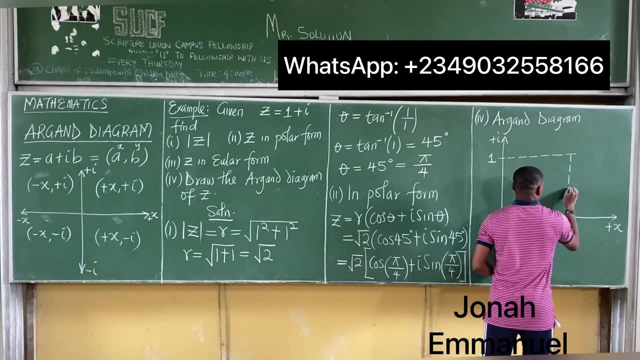 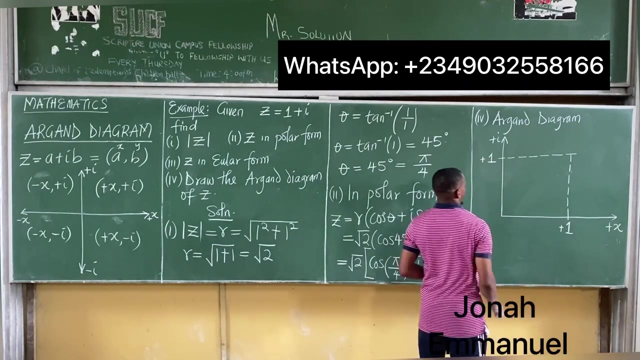 value is one. I'm having one here. it's having one here, so one one, so one. at this point, this is one positive one for the coefficient of I also also I have here as positive one, so positive one, positive one. all right, let's get our line. so a. 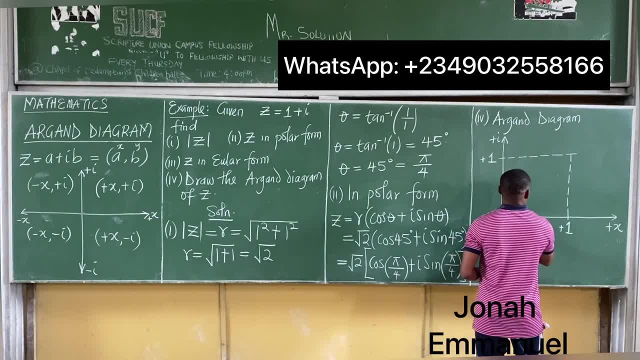 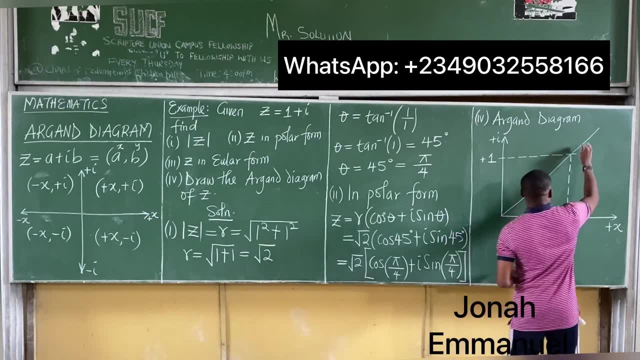 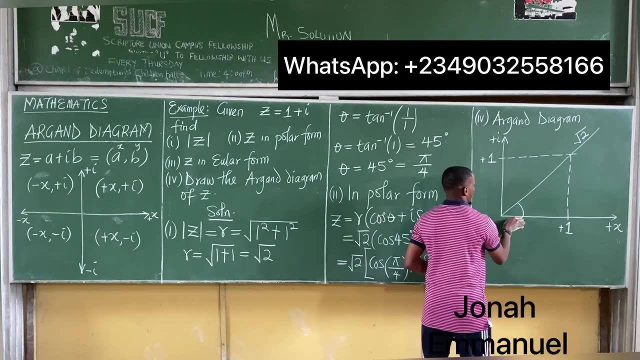 line running from here to that point there something of this nature like this: all right, so that's my, it's in depth. the value here should be R, and we've got now R as root 2, so root 2 will be here. and finally, the angle here, we said, is the. 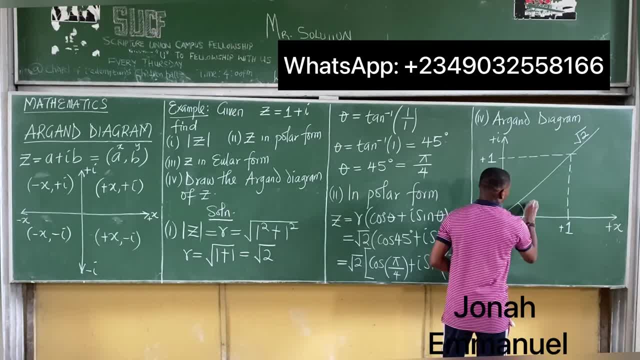 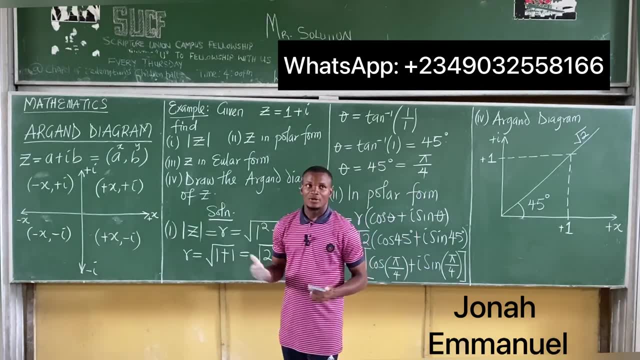 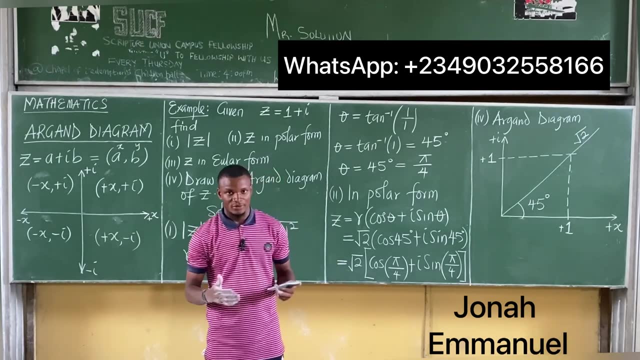 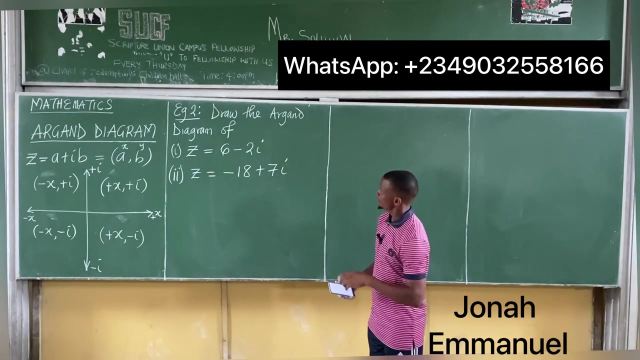 amplitude theta, which we got as 45, so I'm having 45 degrees. so this is how I draw the agand diagram for this question. all right, so this is how I work with argand diagrams in complex numbers. we'll take one last example and we're done with this. so look at a final example on agand diagram. 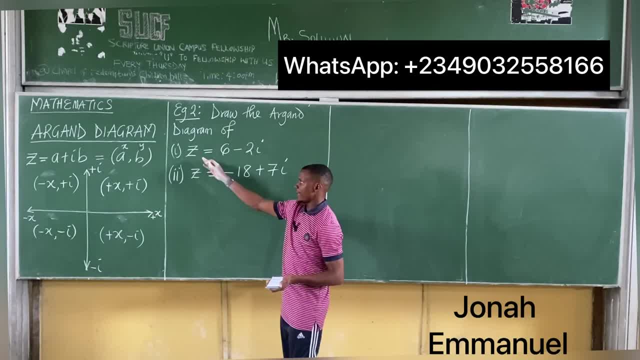 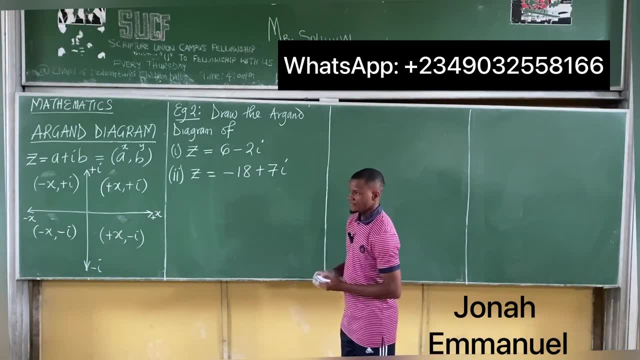 this question says: draw the argand diagram of you have I z being equal to 6 minus 2 I and Ii z equal to minus 18 plus 7i. so I'll do this again in the next three Futures video where you'll see some experimentation between the argument of S. and J coi. you also see that in fugitivefleet and during the rubrics, these two elements as Tr신's elements as TrВО. so this is how we draw the argand diagram for this question, as R equals to role of ui and then D recognizing E drugs. 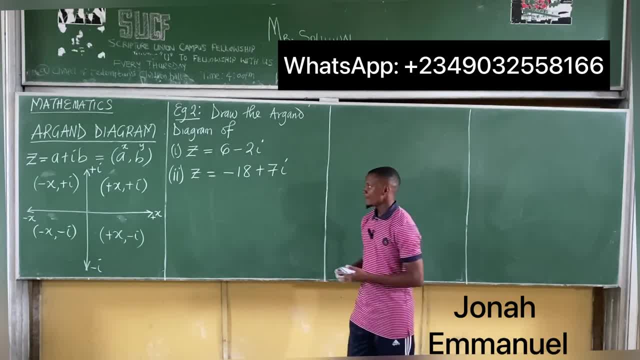 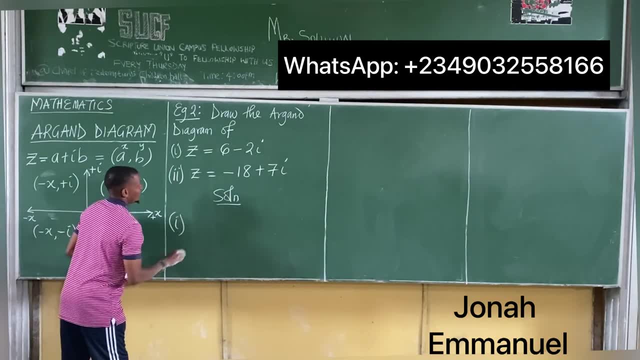 the first part and you attempt the second part. For the first part, solution for i: there I have z being equal to 6 minus 2i. We have this. If I want to get an Erdogan diagram, of course I will need these two values which are given. I also need the value. 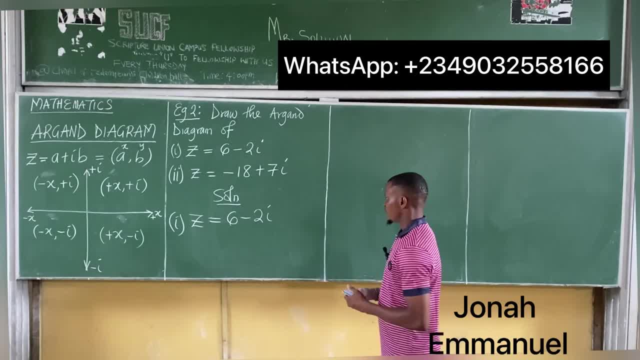 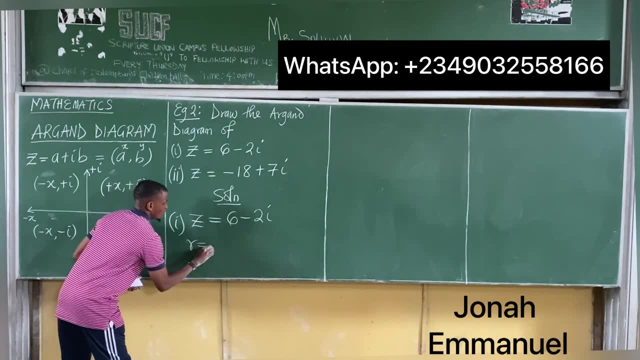 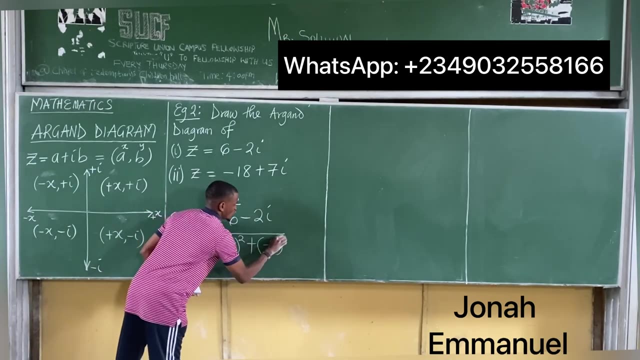 of the modulus and, of course, theta. So let's get the value of the modulus and then theta For this one. here we said the modulus r is equal to the square root of d squared plus 6r squared, plus d squared minus 2r squared. 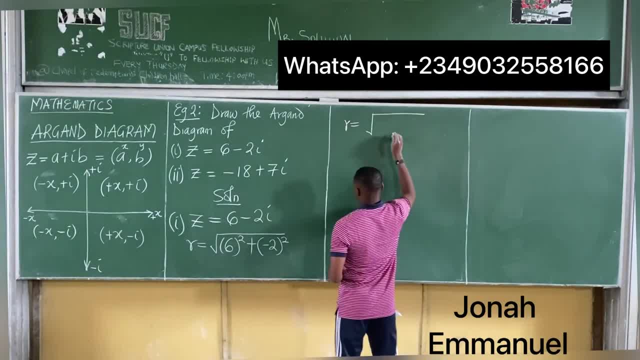 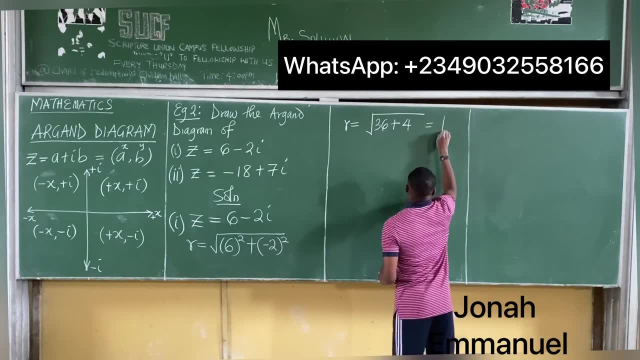 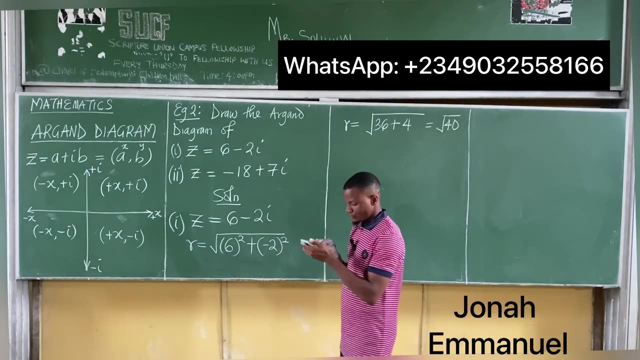 So r is equal to the square root of 6. squared is 36 plus minus 2r squared gives you 4.. That's equal to root 40.. Alright, so that's the value of the r here, Root 40,. can it be broken down? 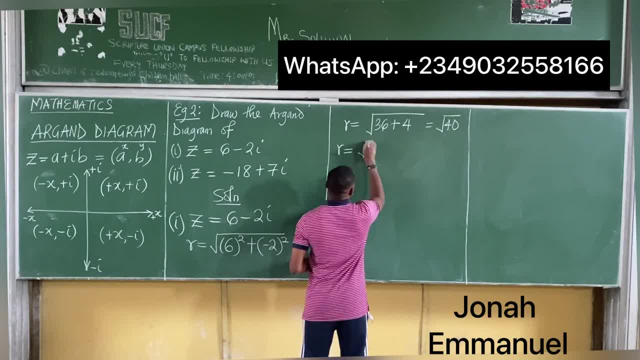 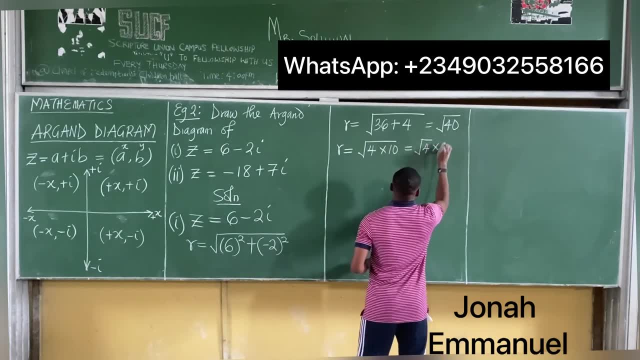 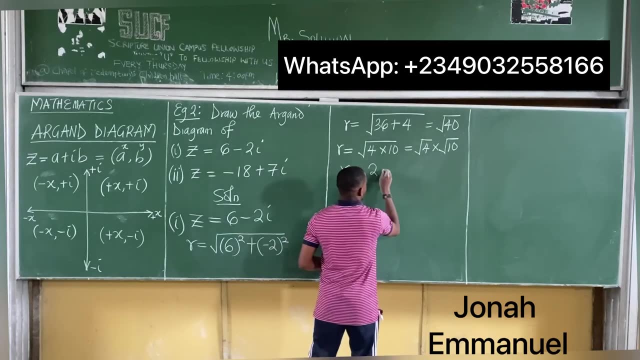 r is equal to root 40 is root 4 times 10.. That's equal to root 4 times root 10.. So r is equal to root 4 is 2 times root 10.. That's 2 root 10.. 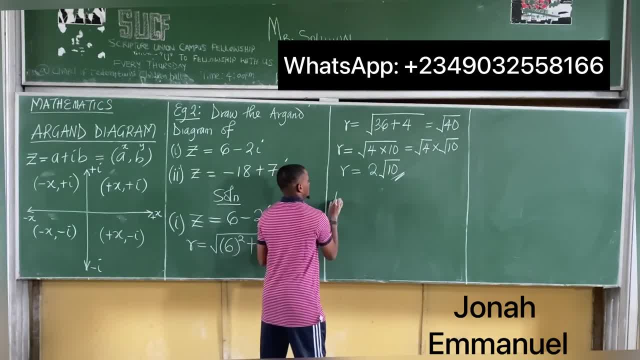 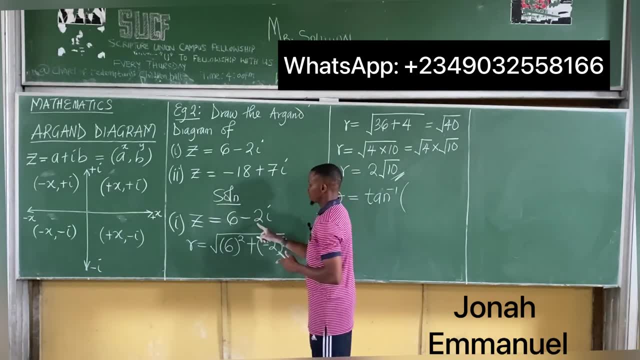 r is 2 root 10.. Let's get theta, the amplitude. Theta, we said, is equal to tan inverse of the b part coefficient of i, which is minus 2.. So minus 2 all over the a part, which is 6.. 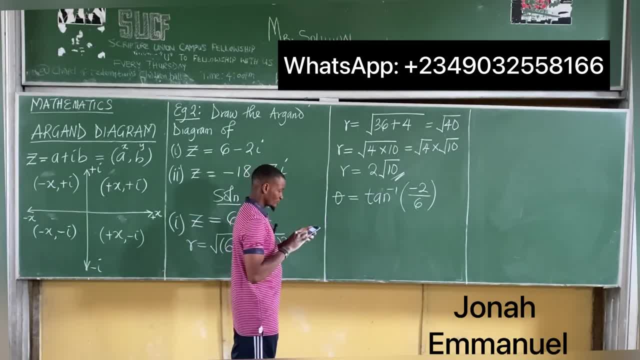 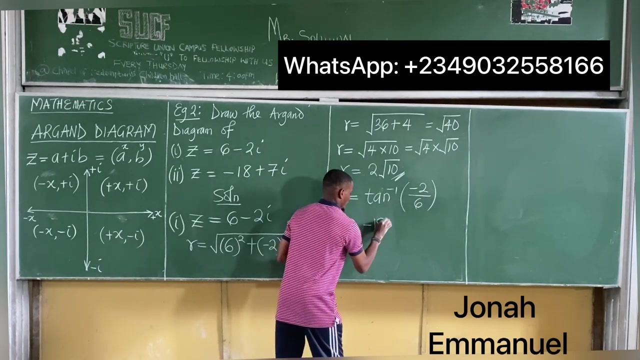 Alright, so let me give my calculator. So I have: theta is equal to tan inverse- I'm punching this directly- tan inverse of minus 2, all over 6. I'm having the answer as I'm having the answer as negative 18 point, negative 18.43 degrees. 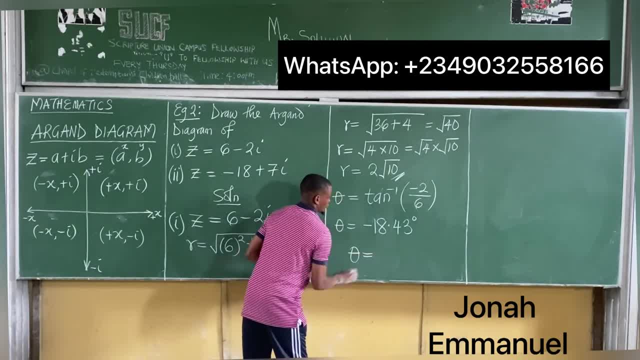 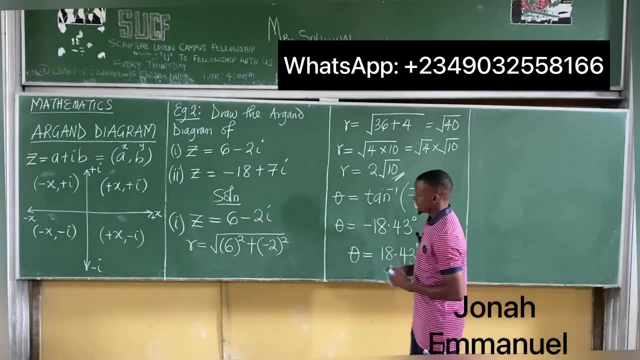 We'll leave out the negative. The negative is only showing direction that is going to be negative. address of the y, It becomes 18.43 degrees. The negative only shows direction That is going to the negative part of I. So finally, my Agand diagram. if I look at this, 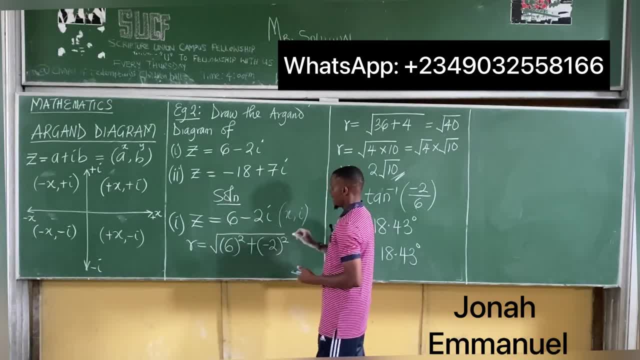 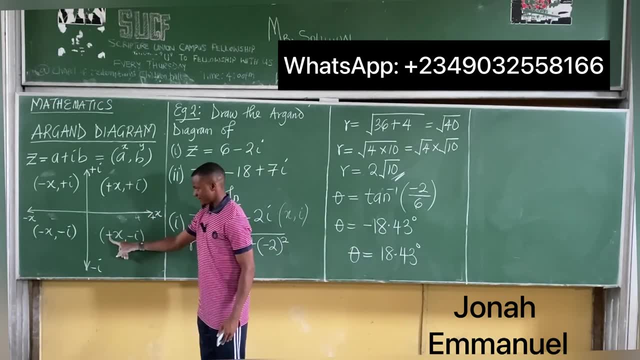 I have remember I said: this is X and I. I have a positive X and a negative I. So if I look at this, it becomes quadrant 4, which is positive X and negative I. So I'll sketch this one here. 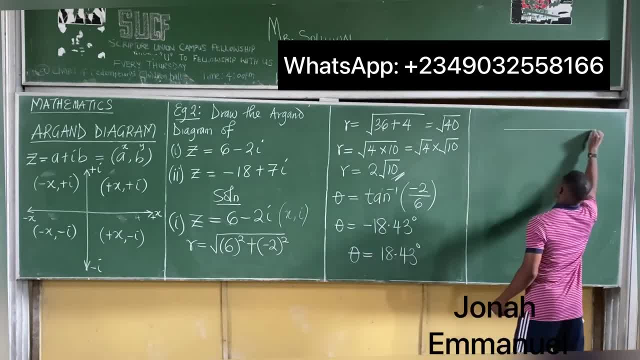 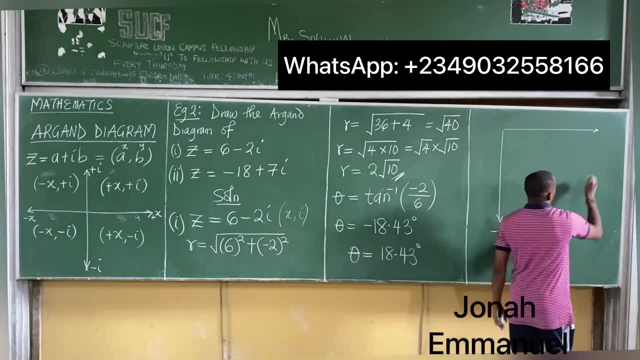 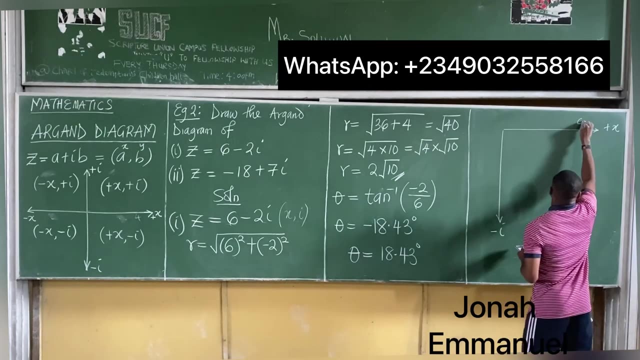 So I'll now sketch this. So my Agand diagram becomes this: positive X and negative I, So I'll label this as negative. I I'll call this as positive X, Negative. I is positive, X is 6.. So somewhere around here I'll call this 6.. 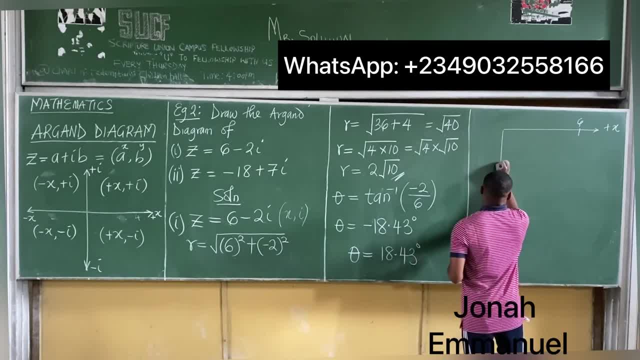 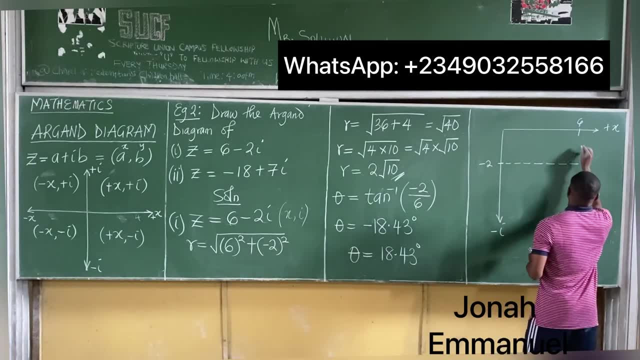 But negative. I is minus 2.. So somewhere around here I'll call this a negative 2.. So look at the point of intersection Here And this one here. So they intersect at this point. So join this to the origin. 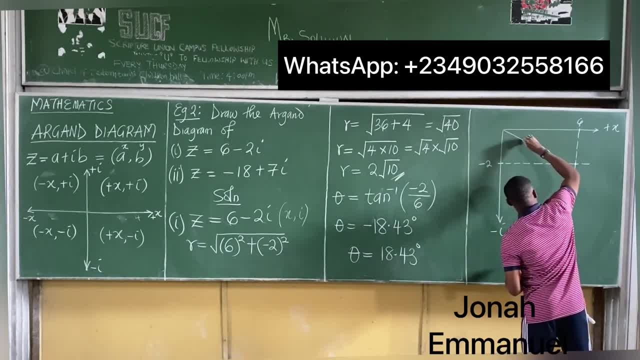 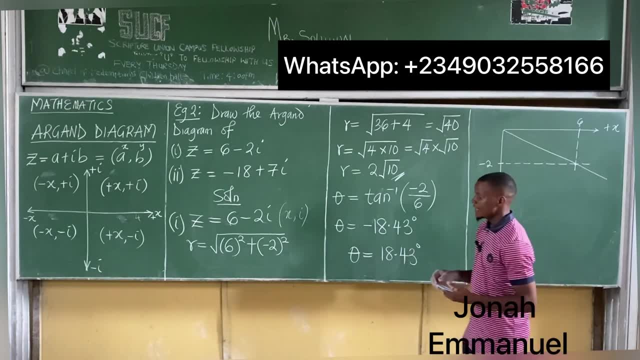 So from my origin, I'll try to join these two. They become this one here, This right, So I have this one here, Alright? The theta is always angle of inclination between R, So this is R. We said R is what there. 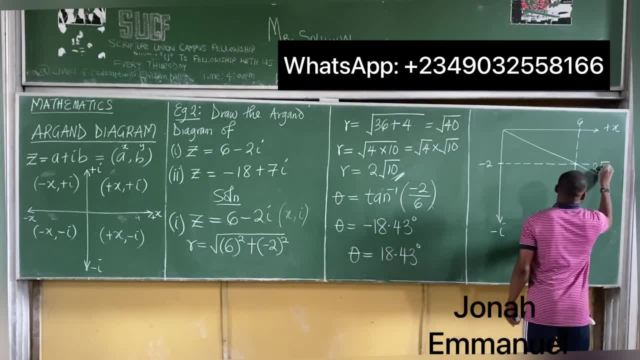 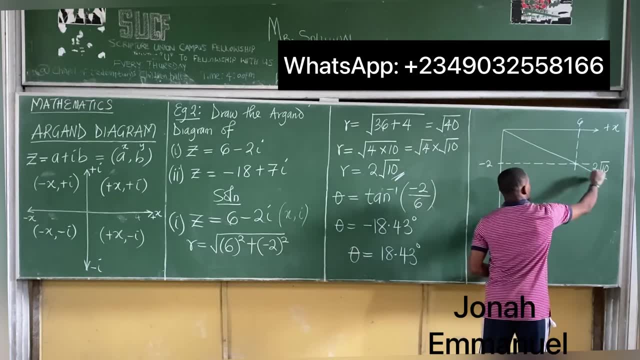 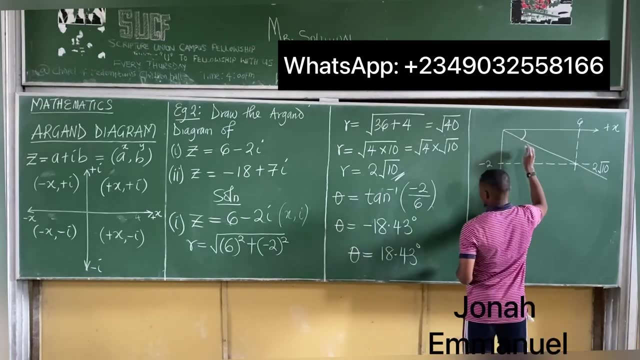 R is 2 root 10.. This is 2 root 10.. This value- here Theta is always angle of inclination between the modulus and the horizontal- becomes this one here. So modulus and horizontal becomes this: This value, we said, is 18.43 degrees. 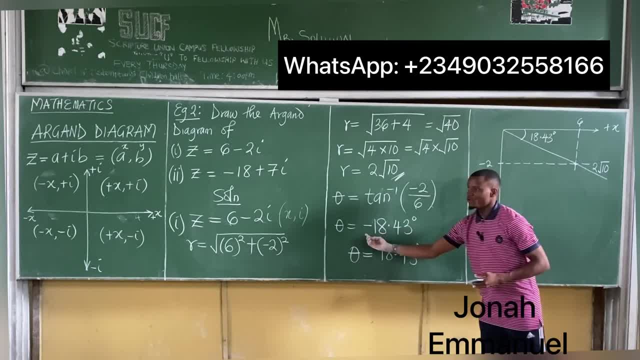 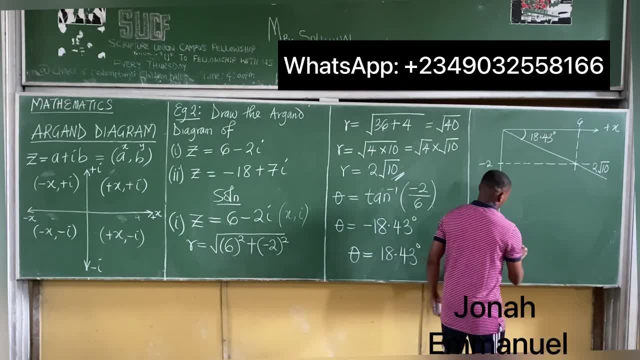 So observe, we took out the minus And I said minus means theta is going to the negative region of I. That's why you have the minus. So I have this as my Argonne diagram. This becomes the Argonne diagram we are required to get. 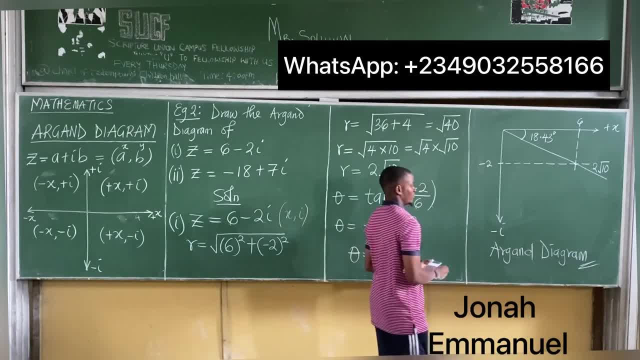 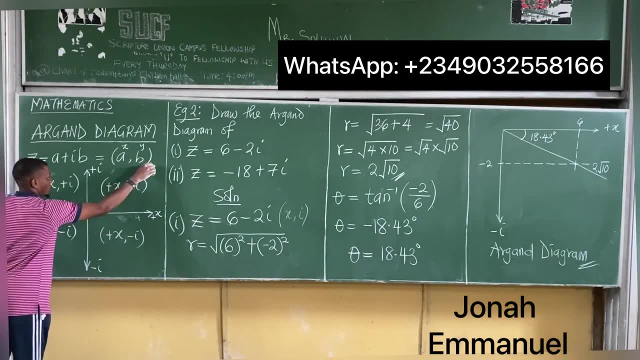 Alright, so that's how we solve this question. Before we leave, please let me show you some things. If I have this one here, I have a line here. Theta will be here. in this case, Theta will be here for quadrant 1.. 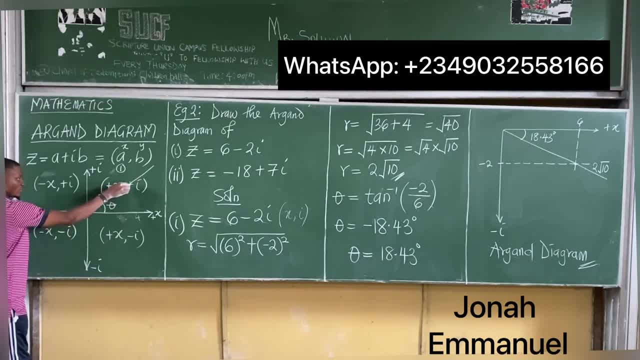 So between the modulus and the horizontal, theta will be here For quadrant 2, if I have a line like this, theta will be this one here. This will be Between the modulus and the horizontal. If I have a quadrant 3 here and I have this line here, 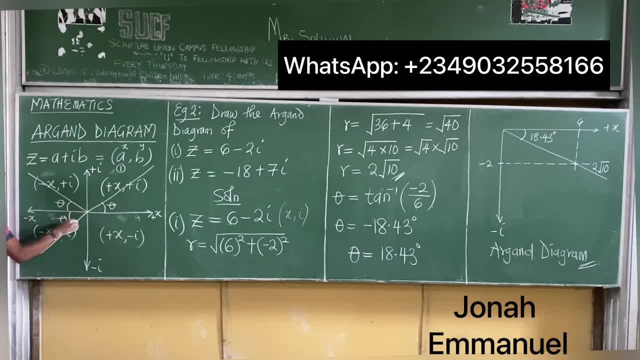 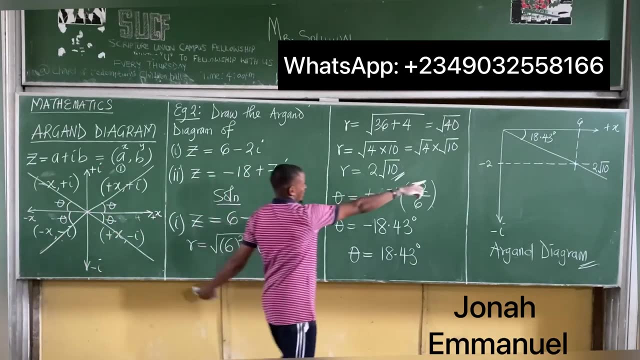 theta will be this way, please: Here Between modulus and horizontal. Finally, for cases of quadrant 4 like this, theta will be here between modulus and horizontal, Just as we have in this case. So see where I place theta here. Alright. 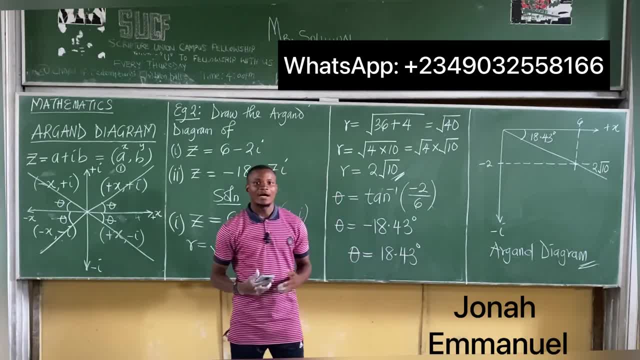 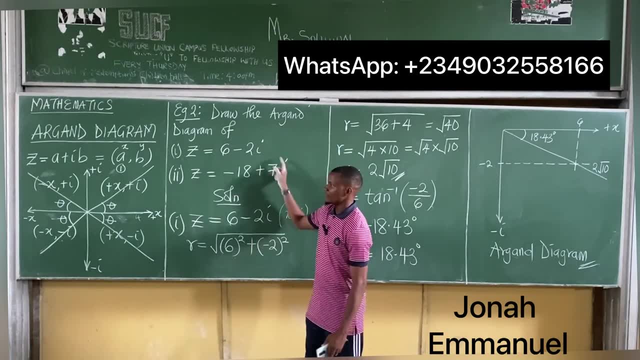 Alright, so this is how we solve problems involving Argand diagram. See you in our next class. Please make sure you do this one here as a trial Test yourself with this, And then, of course, see you in our next class.